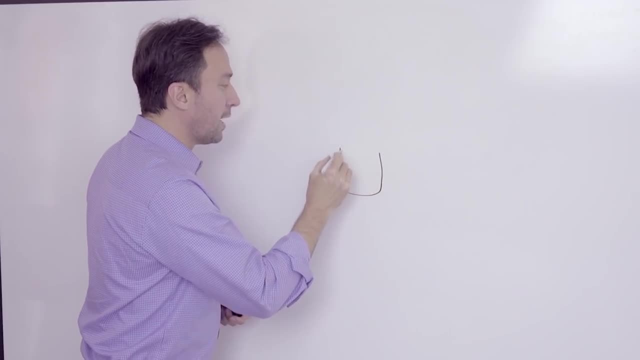 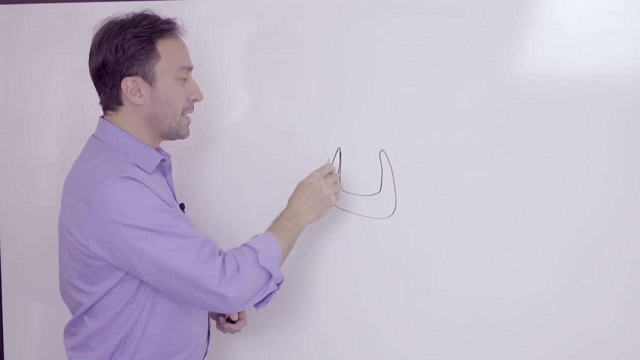 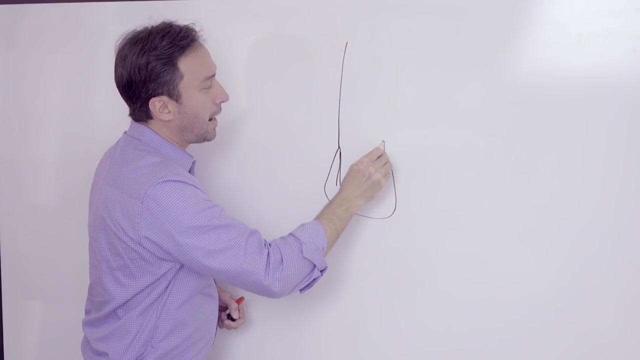 as soon as that is optimized, you have the epithelial root sheath. What this essentially tells us is that the epithelial root sheath, layer D, beer, his very best when Поturigung is. you have the dental cells that are helping you. åºäº, you have the dental cells that are helping you in the uh, in the cap state and the poor- мои. 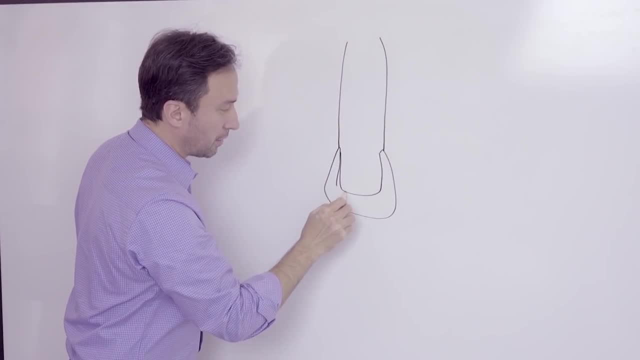 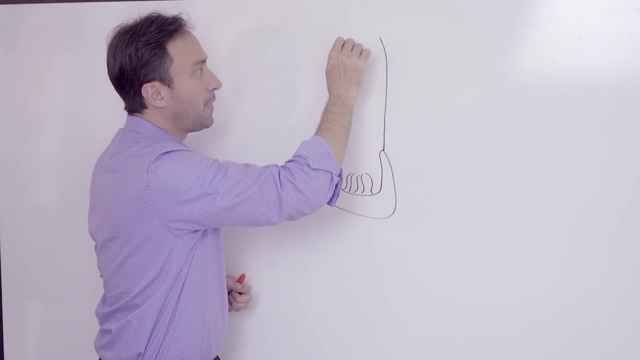 the bell stjet, and then you have your dentinogenesis that triggers your amelogenesis, and then what you, where the enamel is using your odontoblasts and so on, And you end up basically getting a root formation that, once the tooth erupts, the root formation. 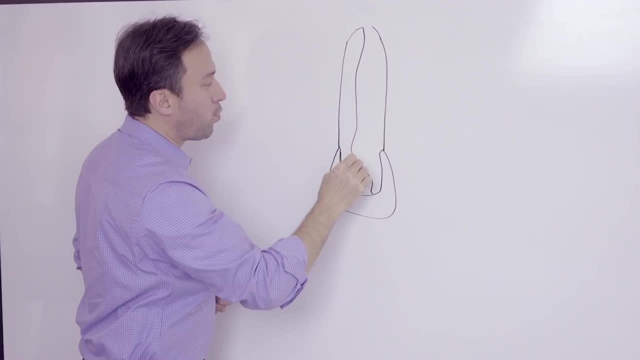 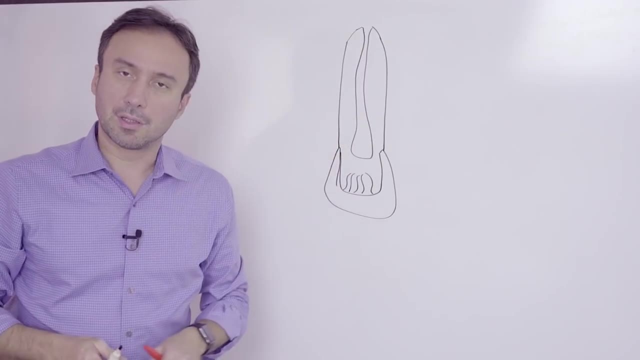 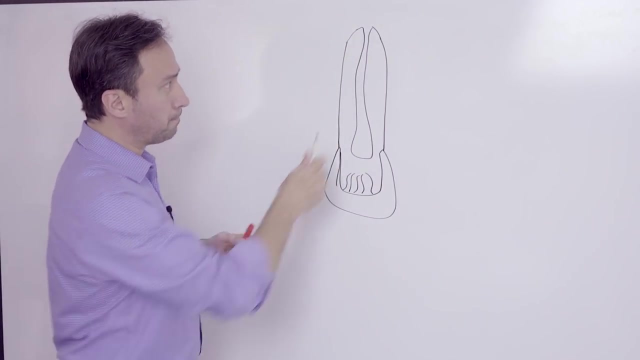 completes a couple of years later on And what you're ending up with is the tissue, that is, the ectomazenchymal tissue that is just adjacent to the dental follicle area, starts to get trapped, as the dentin encloses this ectomazenchymal tissue with the formation of the root. 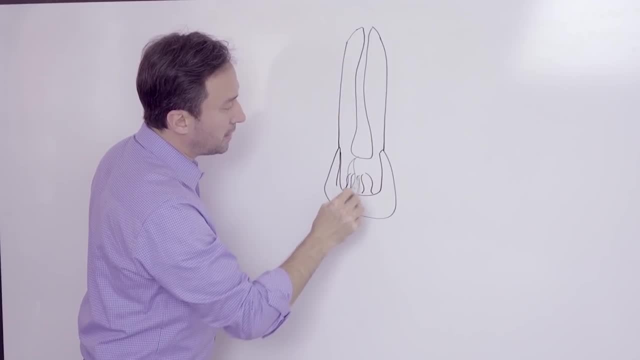 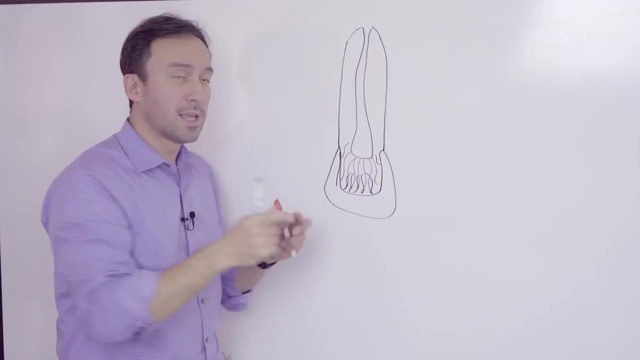 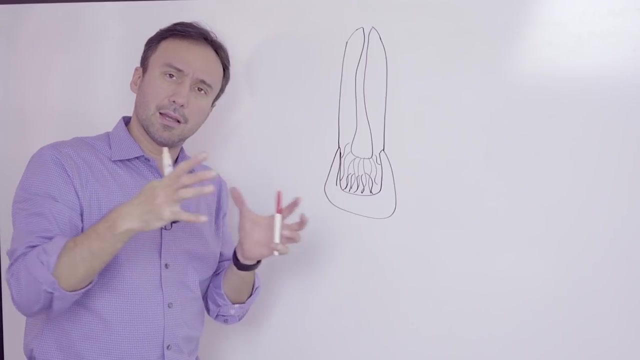 Now the odontoblasts are basically depositing dentin as they're working their way down And obviously, as the dentinal space or the pulpal space starts to get smaller and smaller, the dentin, the odontoblasts, starts to get crunched down. 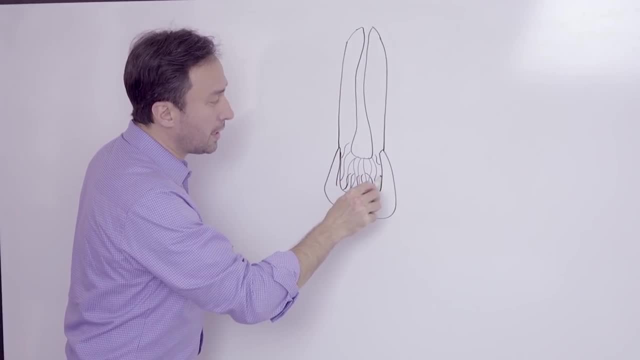 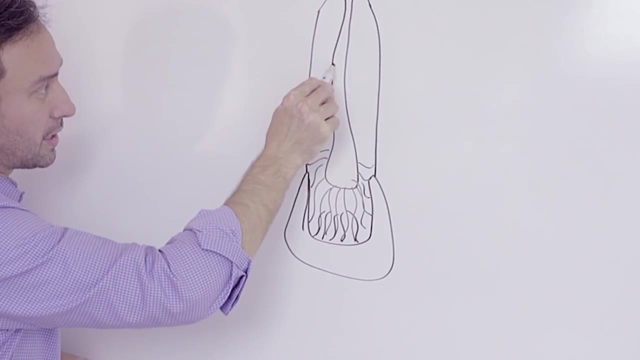 and they get packed into each other, which is the reason why the form of dentin, formation of dental tubules is an S-shape formation to it. Well, first of all, let's just say the composition of the pulp. is you have your odontoblasts? that? 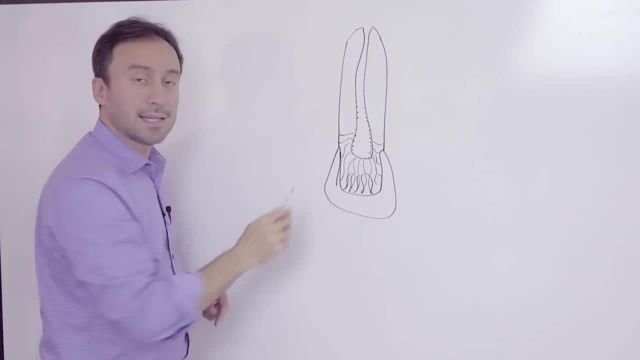 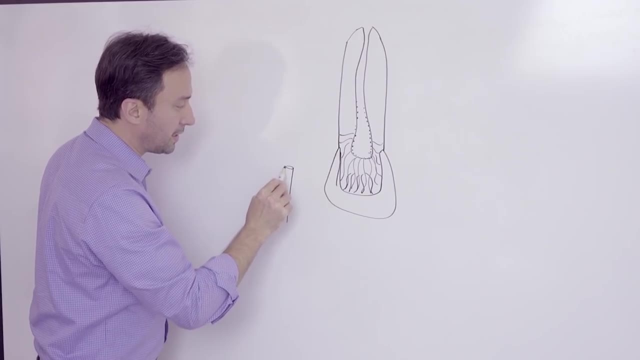 are depositing the dentin, that are lining the dentin, But what's important is, at an ultra-structural level, that the odontoblasts are depositing dentin and you end up having a dental tubule And the dental tubule, which is basically 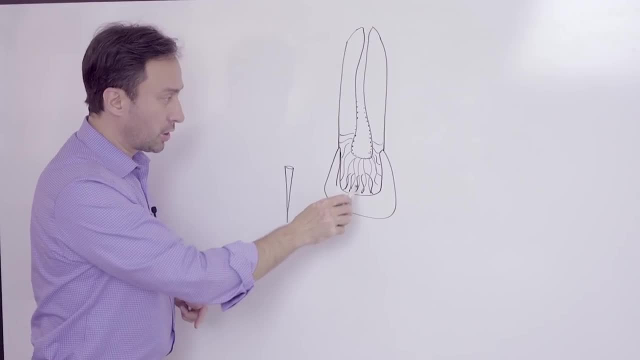 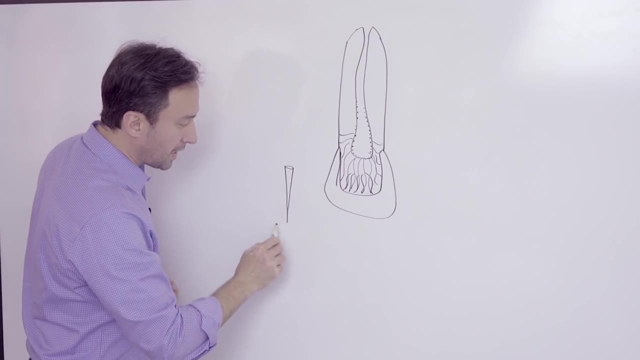 running along from the dentino-enamel junction all the way to the pulpal surface, is conical in shape, ultra-structurally, And what it is that? if you look at the dental enamel junction portion of it right over here, the diameter of these tubules, 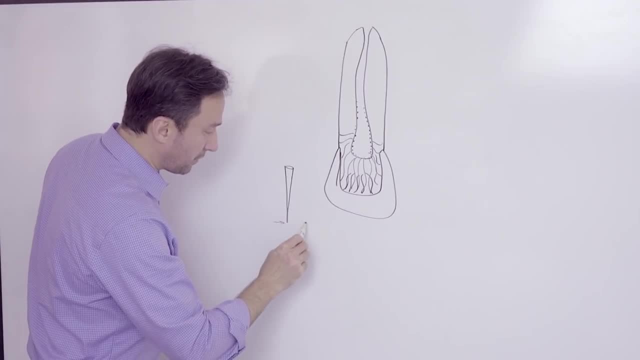 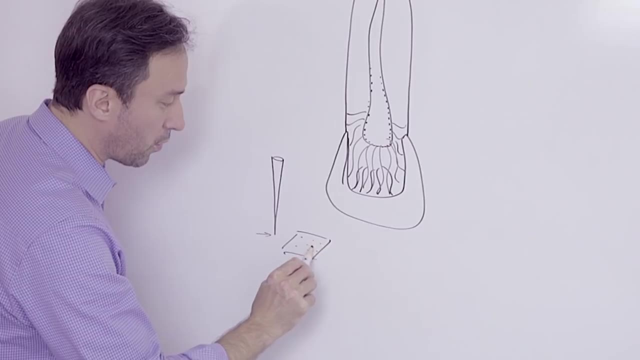 are somewhere around one micron or less, And what it means is that if you take a histological section here, you take a look at the dentin in a square area, you're having basically somewhere around 1% of the surface of the dentin at the dental enamel junction. 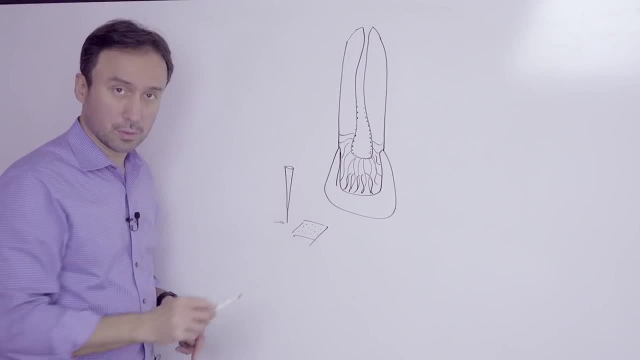 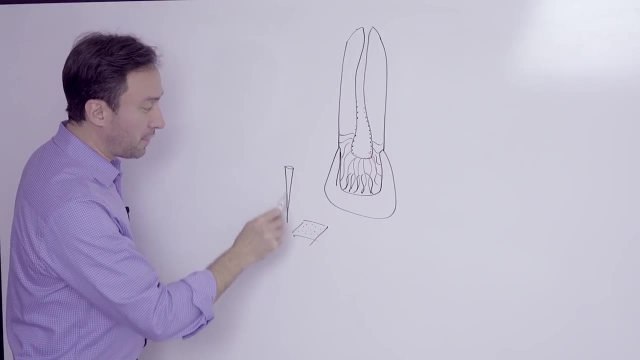 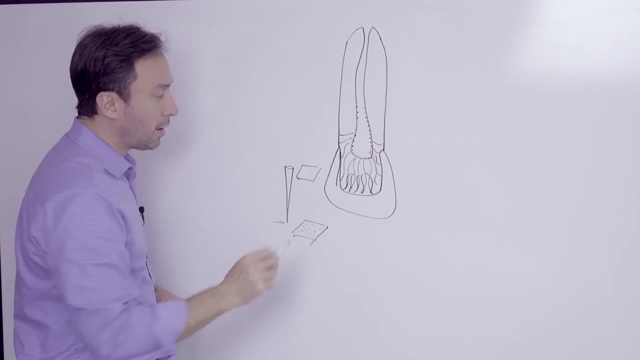 is tubular. That is the diameter of the tubules. So you only have 1% density of the tubules in that area of dentin. But if you go all the way up here at the pulpal surface, all of a sudden you take a cross section of that per square area. 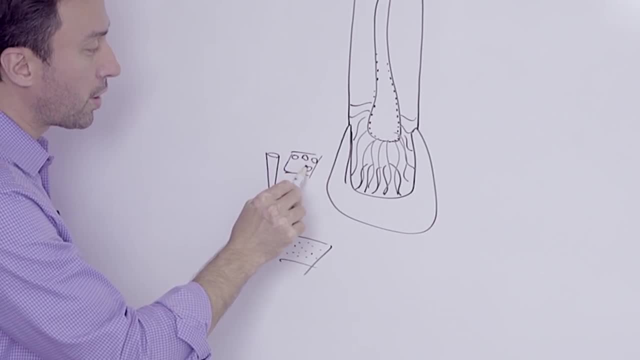 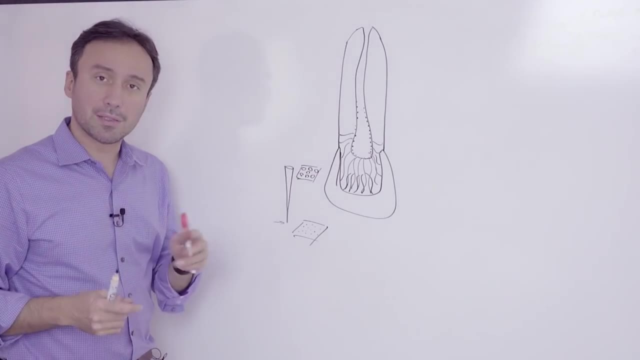 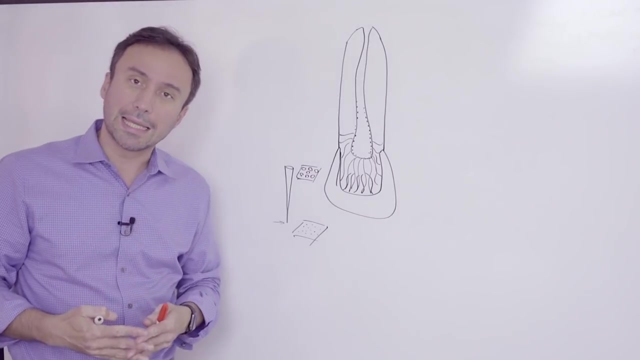 you're having somewhere closer to 40,. in some cases, even 50% of the surface of the dentin is occupied by these tubules. What does that mean? So what that means is that dentin starts to have increased permeability as you go deeper. 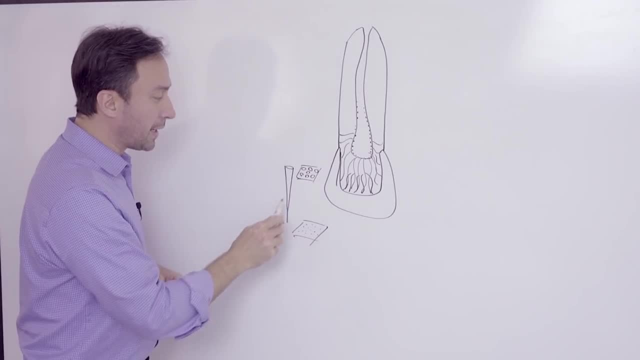 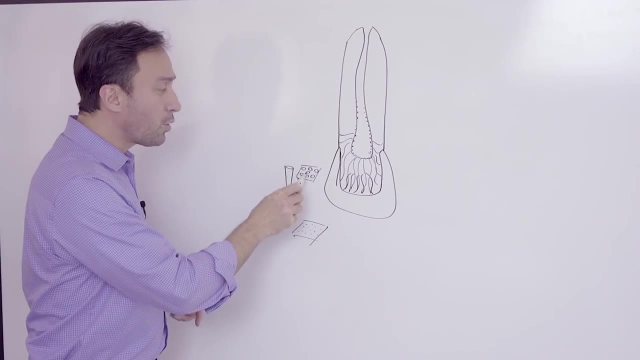 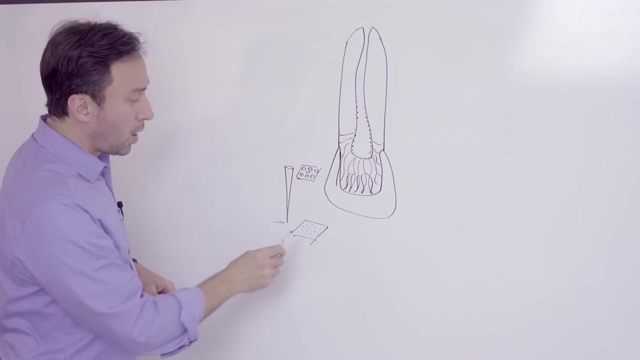 and you get closer to the pulp And, as a result, what ends up happening is that, as decay as well as our fillings end up getting deeper, now you have a higher chance of leakage through dentin into the pulp. that causes contamination. So, while the diameter here is about 1% and one micron and less, 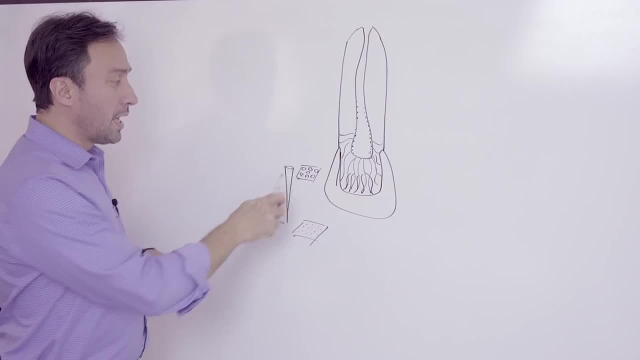 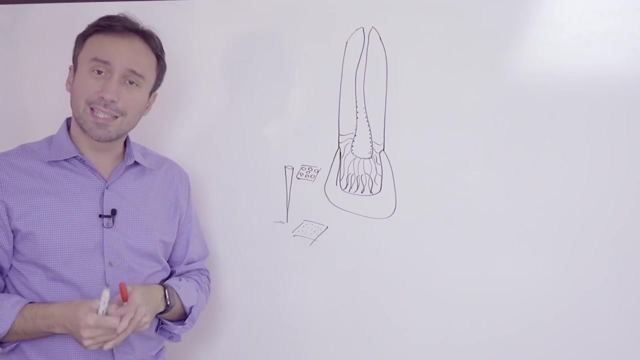 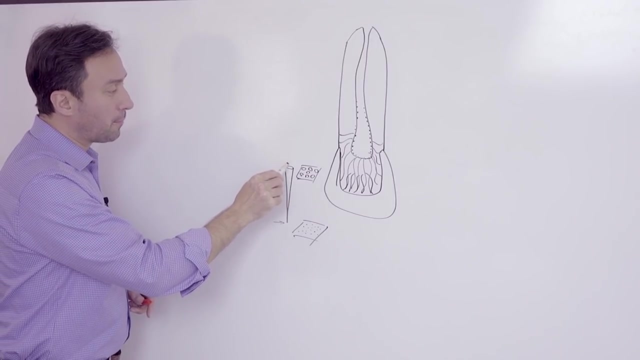 so it's fairly closed off. the deeper you go, it gets more permeable, So that is really the reason why you can have a higher chance of infection, as well as more sensitivity, the deeper you go towards the pulp And, naturally speaking, you have your odontoblasts in here. 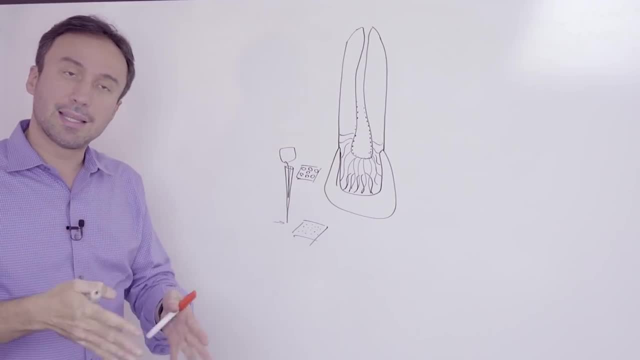 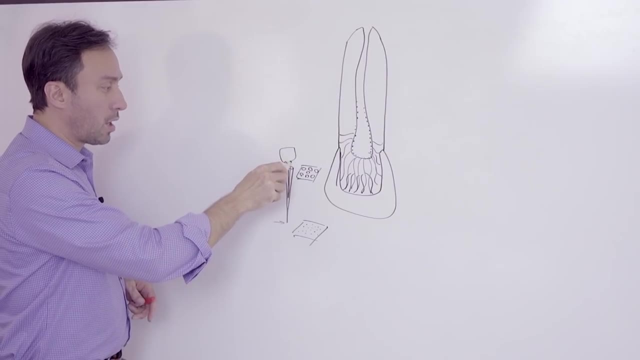 And there's an odontoblast process that is extended into the dental tubule. In fact, that's how the tubule is formed, as the process the odontoblasts- Yeah, The odontoblast process- deposits the peritubular dentin. 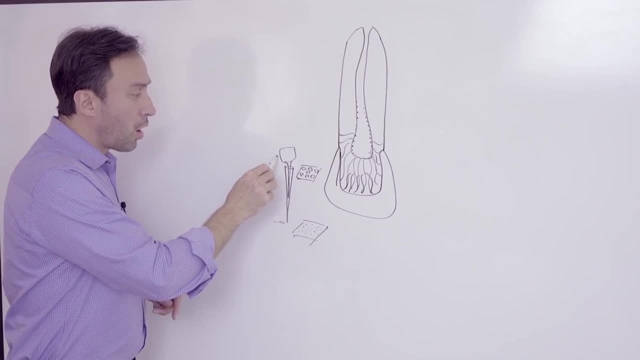 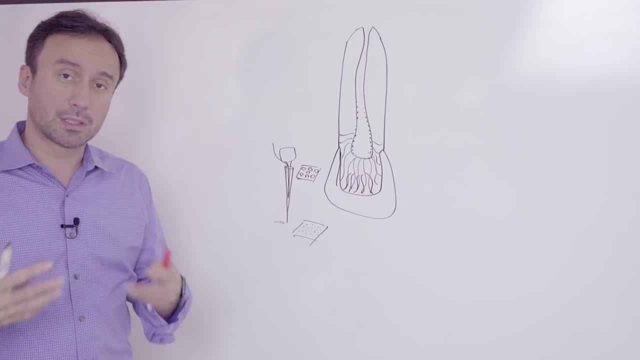 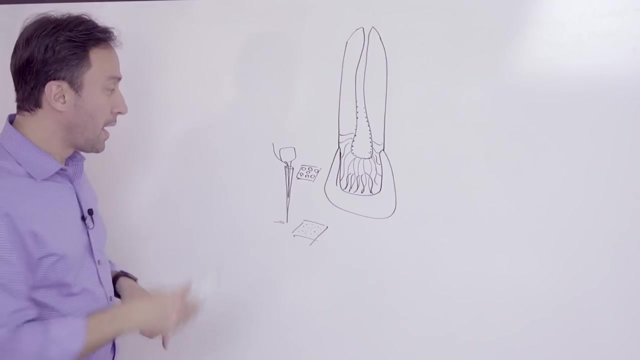 and so on. But there is also a nerve fiber that goes inside here as well, that gives innervation to the dentin And that's what creates the dentin pulp complex and the reason why our dentin has sensation. Now it's important to understand. 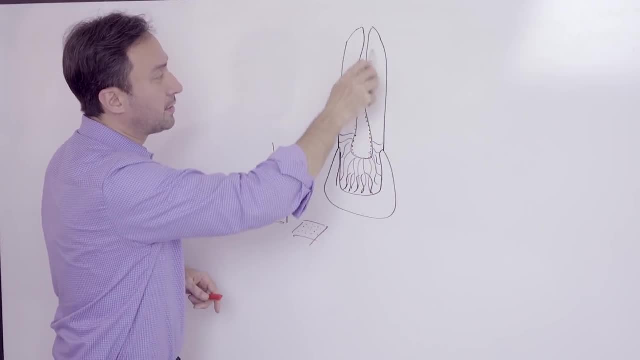 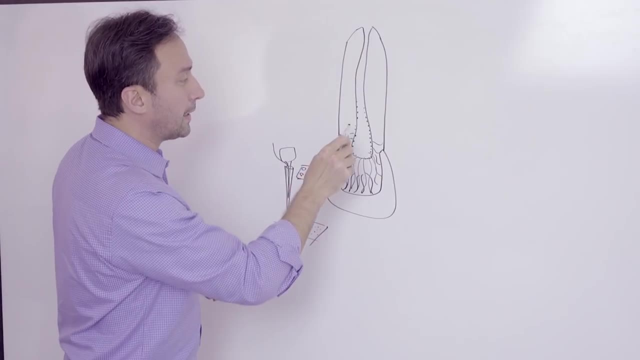 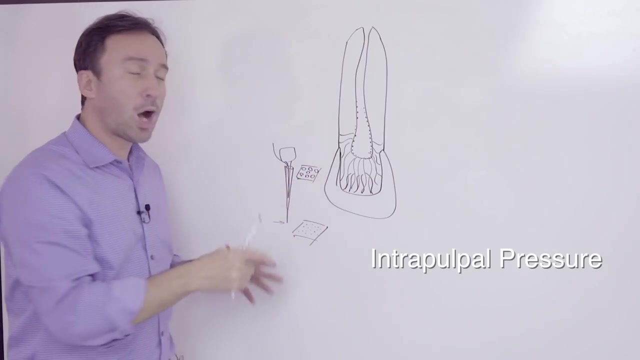 that, as we mentioned, this area gets closed off and the pulpal tissue gets encased. There is a certain amount of pulpal pressure that is present inside this space And, as a result of this pulpal pressure, there is an outward flow of fluids. 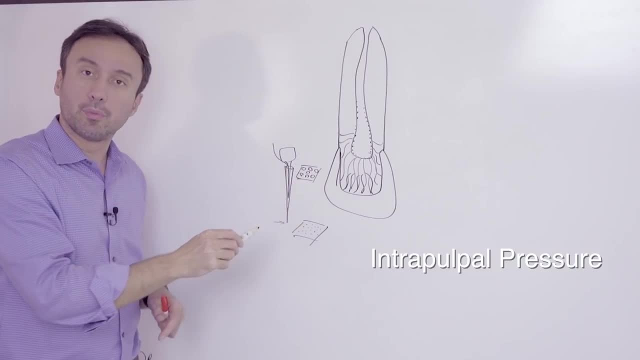 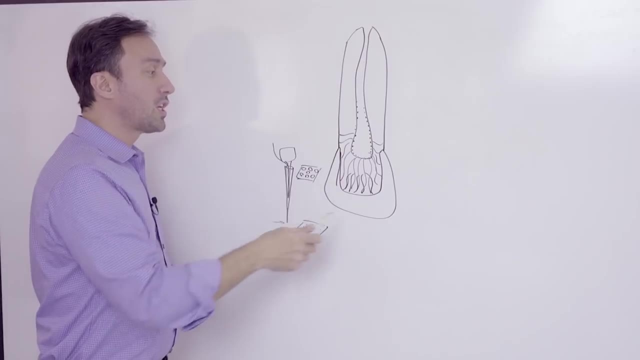 which is interstitial fluid inside this dental tubule. So this dental tubule is constantly being flushed out. That is an evolutionary process by which we don't just keep on getting infections, because the dental tubule is constantly being flushed out And that's a 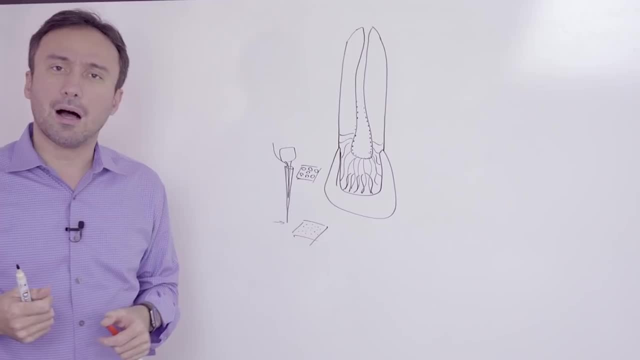 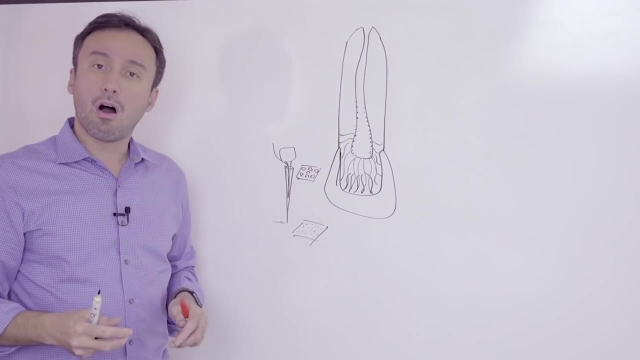 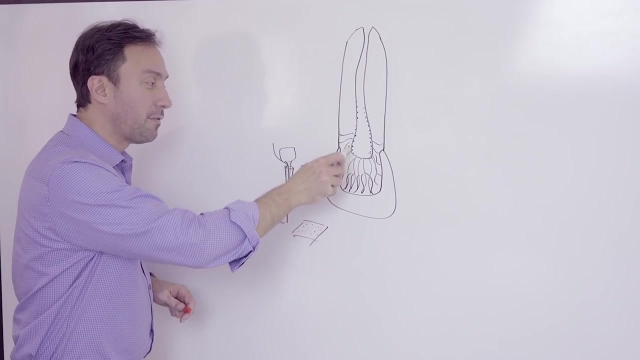 That is a property of live dentin that has a flushing mechanism. In fact, if you do a crown prep and you cut your crown and you let your tooth sit there after a while, you get a phenomenon called dentinal sweating And what that is is basically the flushing. 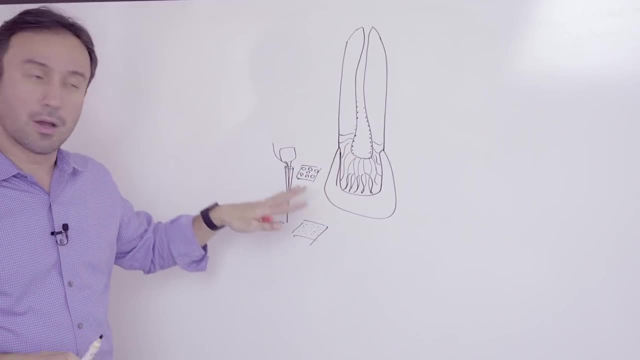 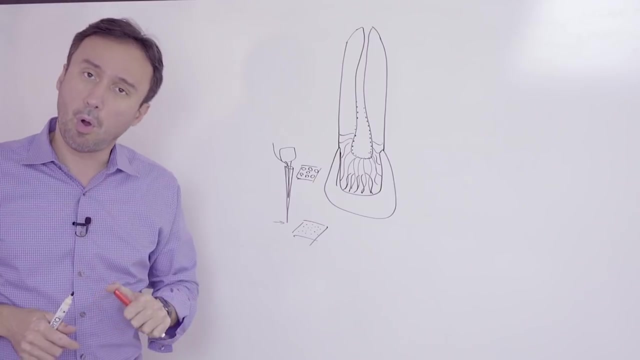 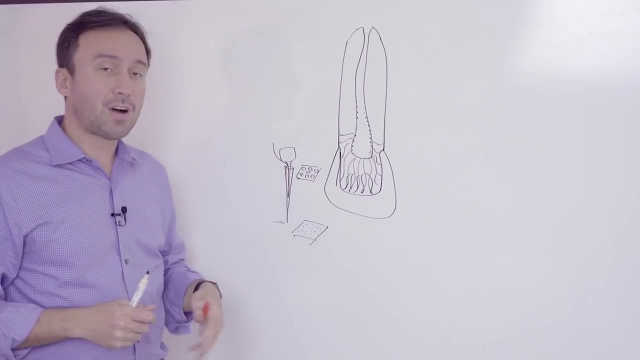 of the dental tubules with the interstitial fluid, which is intratubular fluid inside the tubules. that hopefully keeps it clean and prevents contamination of the pulp, which is also another reason why dentinal tubules that are devitalized or, in the case of a root canal, treated tooth. 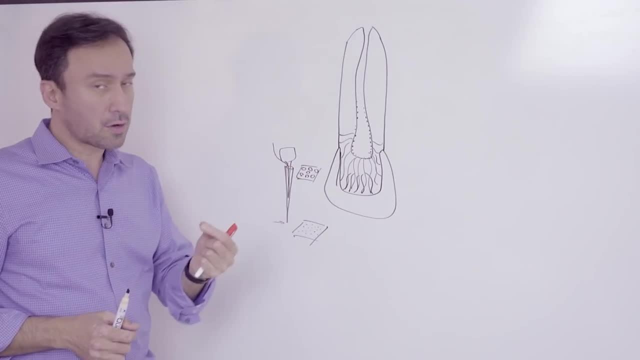 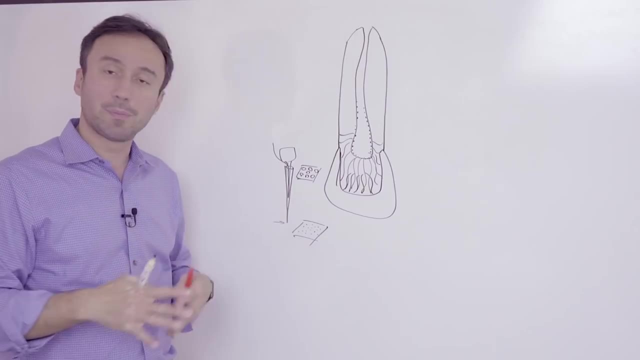 the permeability of dentin is increased, which is another reason why, from a clinically significant point of view, all devitalized teeth should be covered. The dentin should be covered. So if you do a root canal on a tooth because there's no sensation, it doesn't. 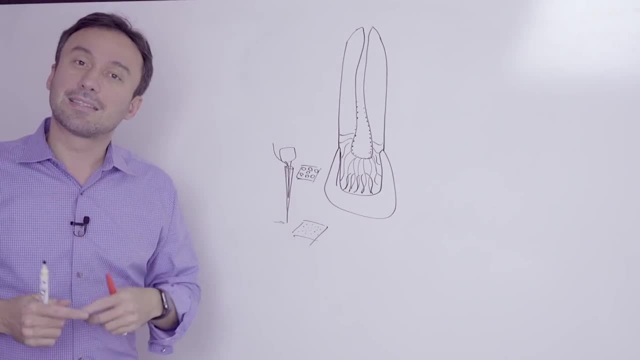 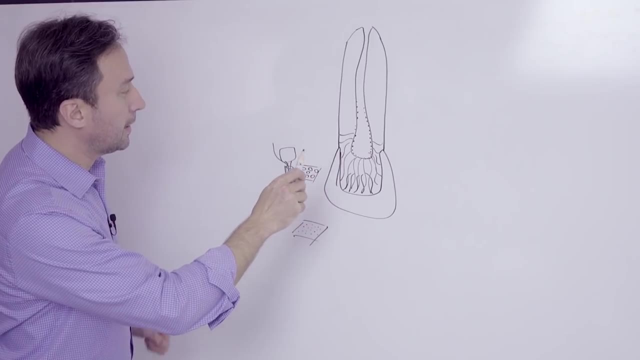 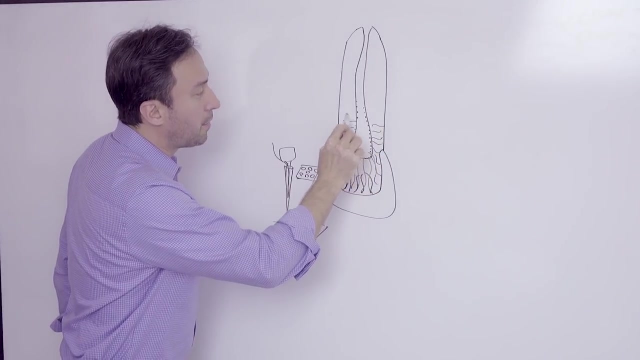 mean that you can just leave the crown off because that dentin is going to be permeable, So So it should be covered. Anyway, that was just another clinical little tip here. But what we need to realize is that the dental tubules end up. 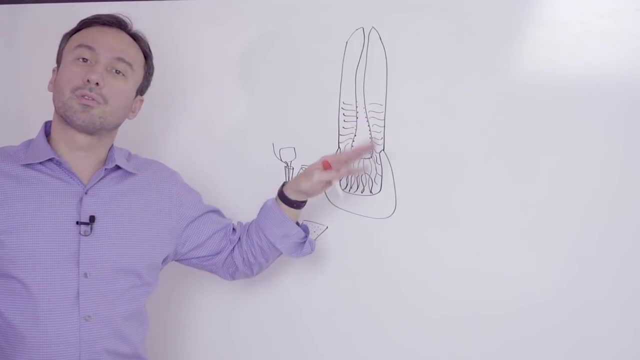 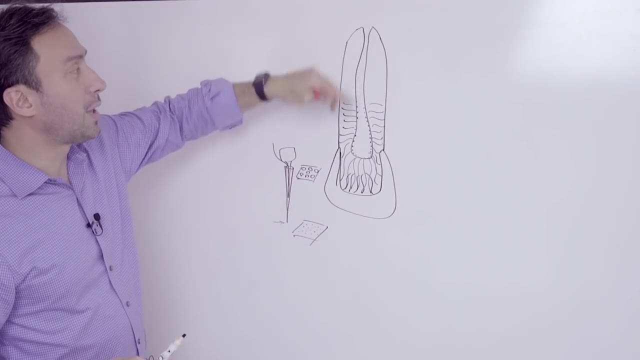 getting more and more amorphous the closer you get to the apex, So that the upper half of the coronal half of the root has dental tubules in it, but the apical half, and specifically the apical 1 third of the root, 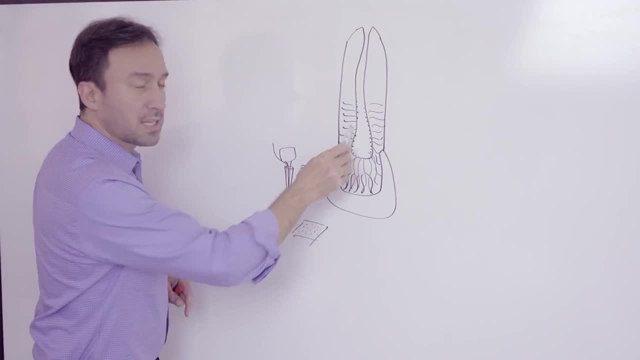 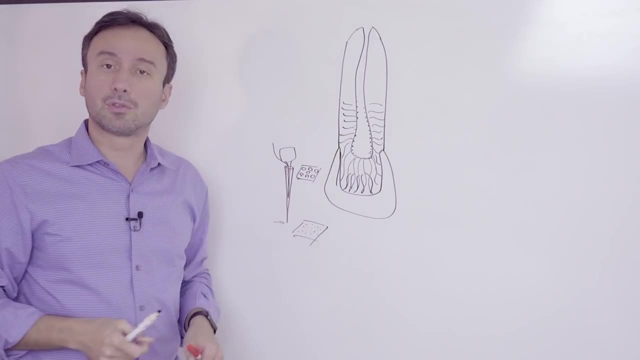 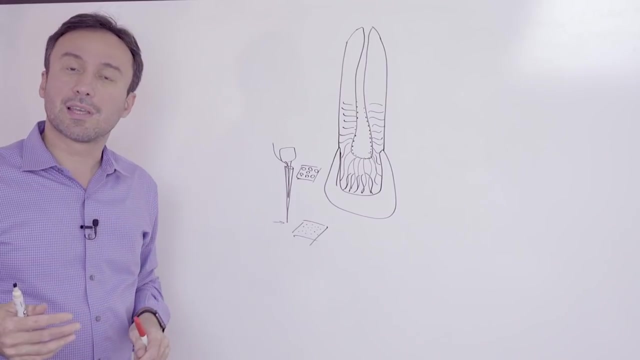 has amorphous dentin And so This is significant because we know the use of composites for mechanical bonding is important where you have dental tubules. So we know that we don't have that in the apical half, which is the reason why resin bonded restorations and any 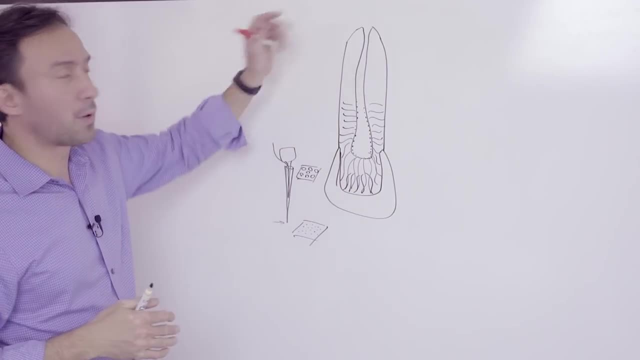 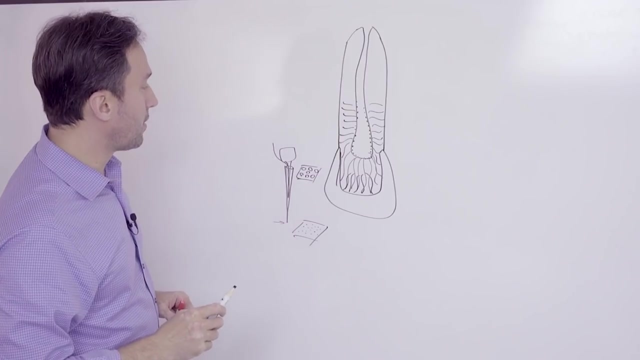 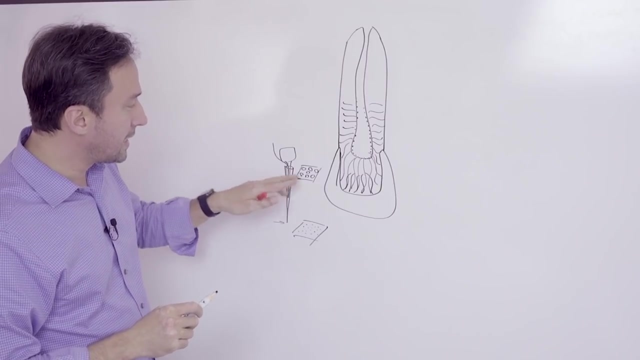 of that resin. mechanical bonding is ineffective in the apical half of the root, And that's only good in the coronal half, OK. So that's another piece of significance to realize that. But another thing that we need to know is that it's the movement of the fluids. 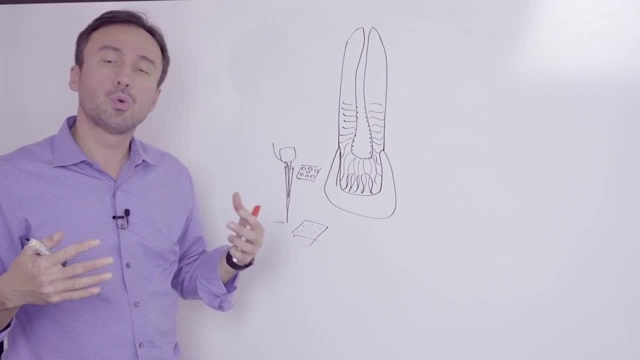 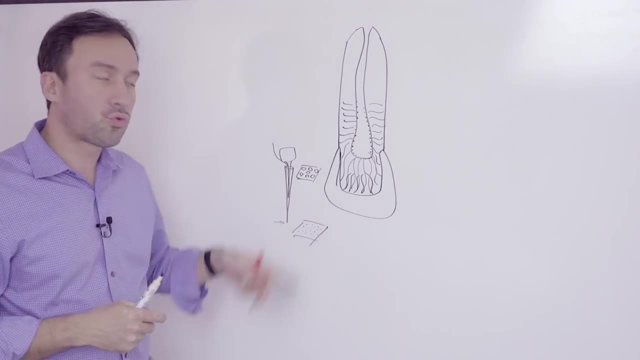 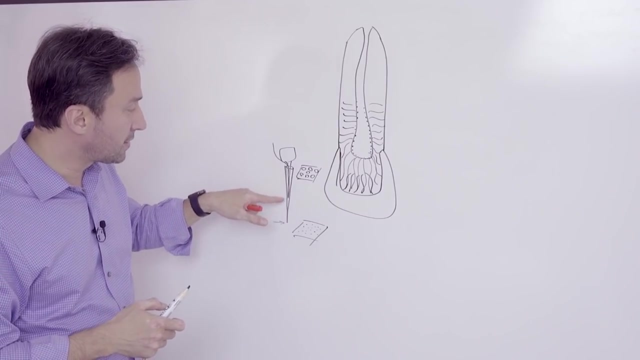 As I mentioned, there is a gentle outward flow to the fluids in the dental tubules that is constantly present. However, any rapid increase in the rate of outward flow of the fluid is what triggers the nerve that is inside the dental tubules And that triggers a sharp shooting pain to the patient. 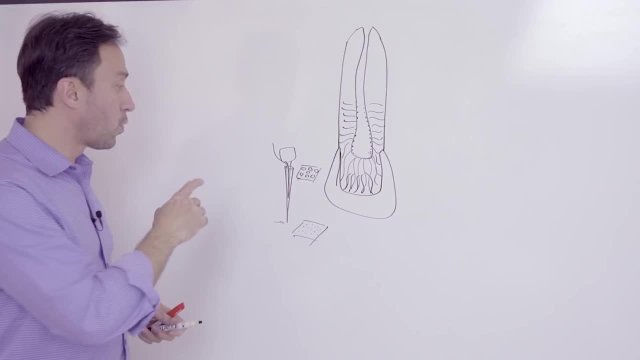 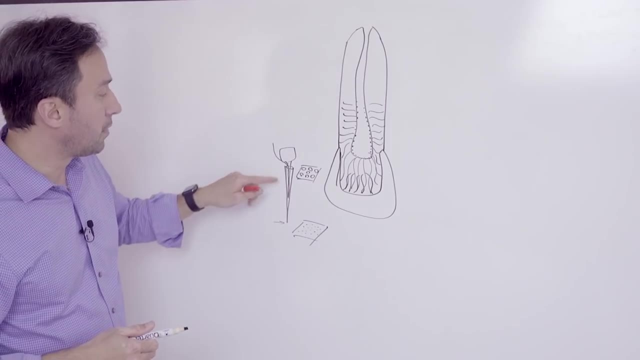 That is the mechanism of dental sensitivity And why, If you were to actually run your explorer over live dentin, the patient will actually have a sensation, And that's as a result of the movement of the fluids in the dental tubule. OK, 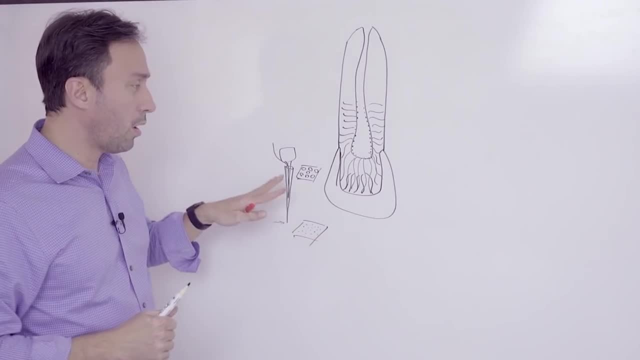 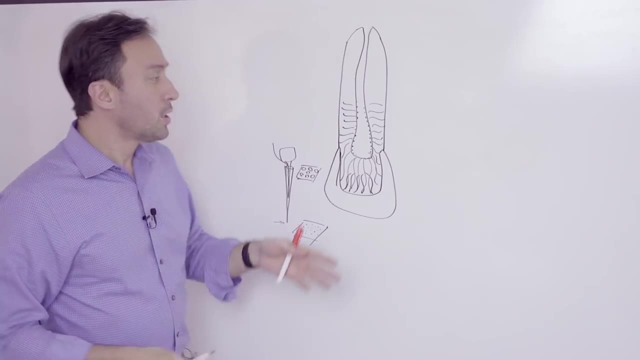 So now that we're talking about the innervation and the nerve that's in the dental tubules, it's important to also talk about the neurovascular bundle and the way it enters the pulp. So your most numerous cells inside your pulp is your fibroblasts. 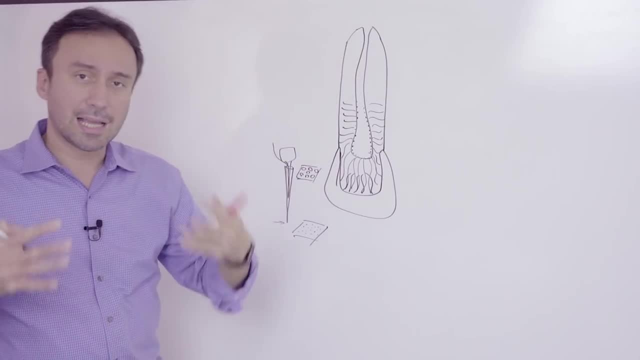 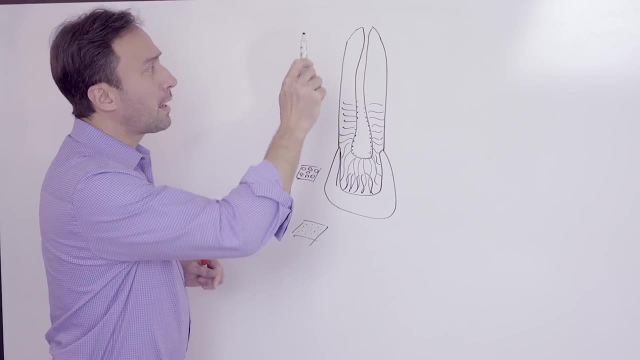 As well As, obviously, then you have your specialized, this highly specialized the oloblasts that are present in there and a number of other cells. But what about vasculature and the neurovascular bundle? Well, we all know that, from an anatomical point of view, as this tissue gets trapped, it also traps in a neurovascular bundle that will innervate as well as nourish or give vitality to the pulp. So For the vascular component, the highest level of vascularity is provided by venules as well as by arterioles. 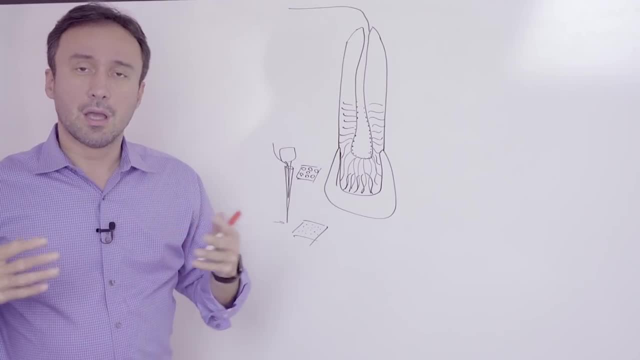 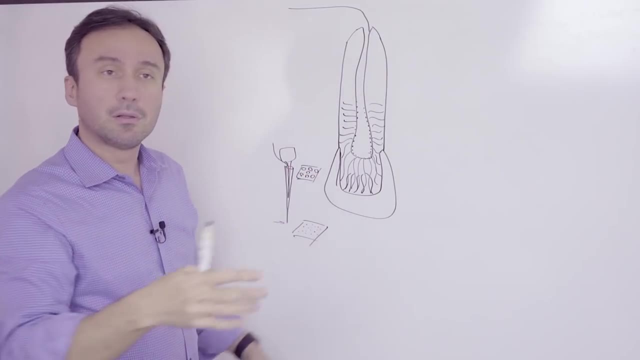 So there are no arteries or veins, but we're talking about venules and arterioles. But what about innervation? Well, for innervation we're talking about on the maxillary branches of the trigeminal V2 branches. 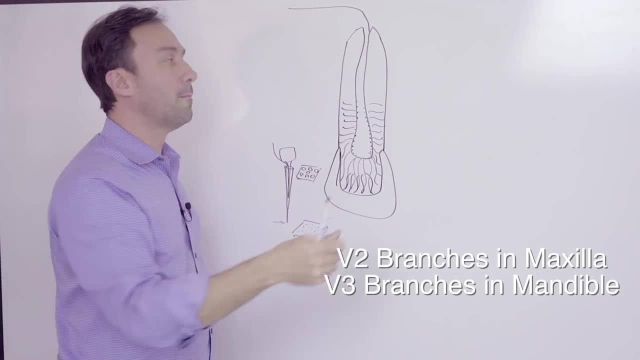 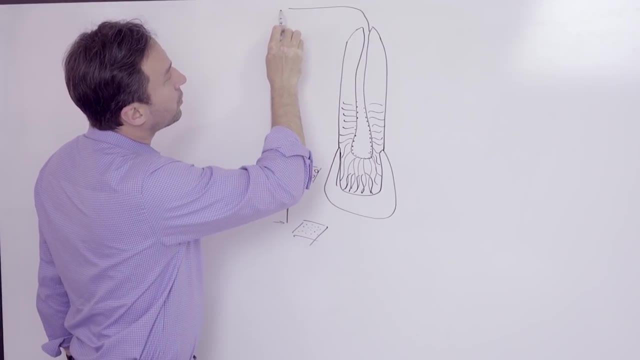 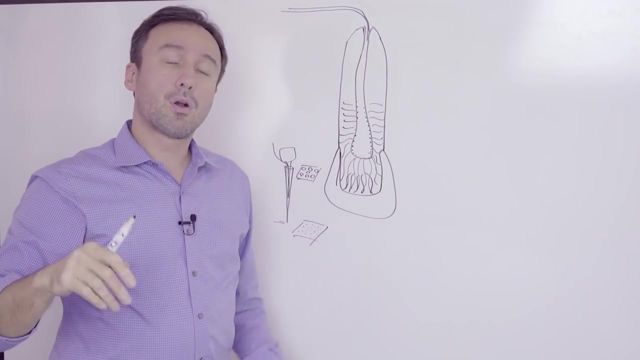 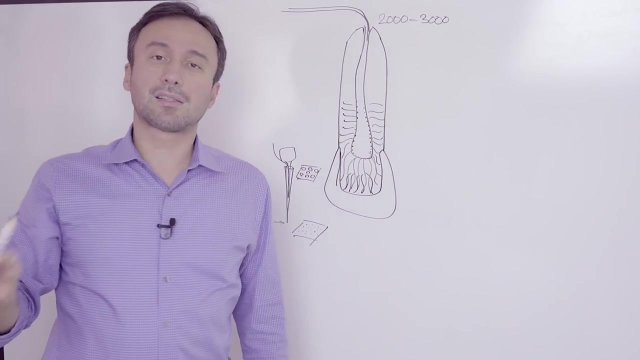 For innervation. we have primarily afferent, sensory afferent nerves as well as some autonomic branches, But we have your axons of the nerve through the V2 coming in and branching and getting inside the pulp. Now there are only about 2,000 to 3,000 individual axons. 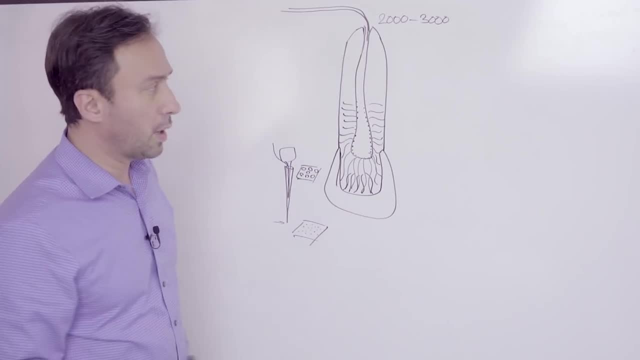 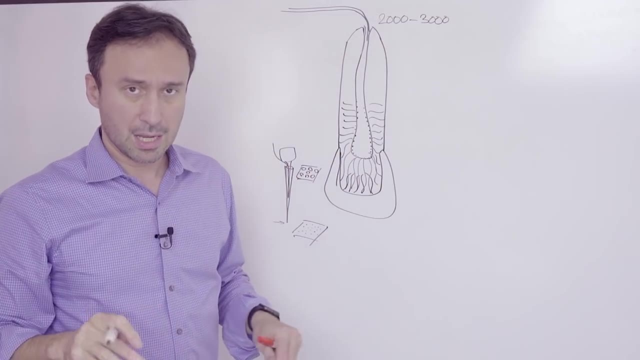 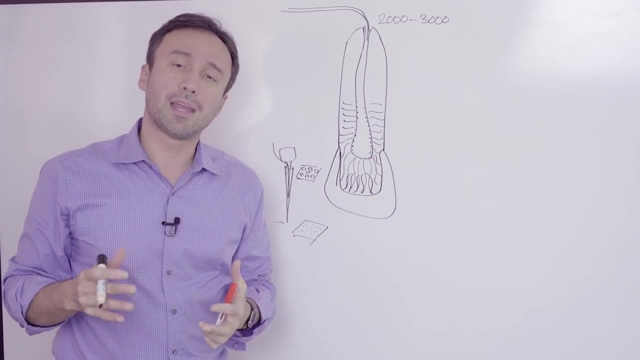 that enter the pulp of a tooth- each pulp if you will- And these are basically categorized in specific ways And I'm going to talk to you about them in a moment. But it's important to realize that understanding this innervation will give you a wealth of information. 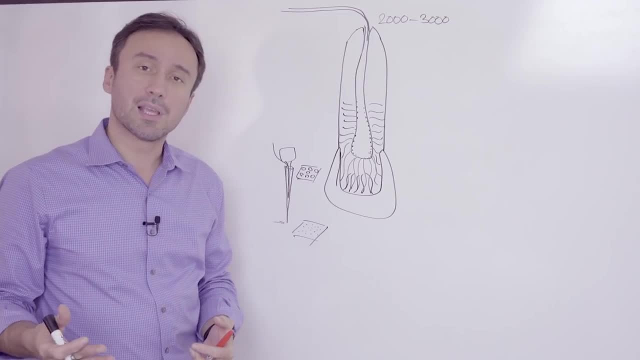 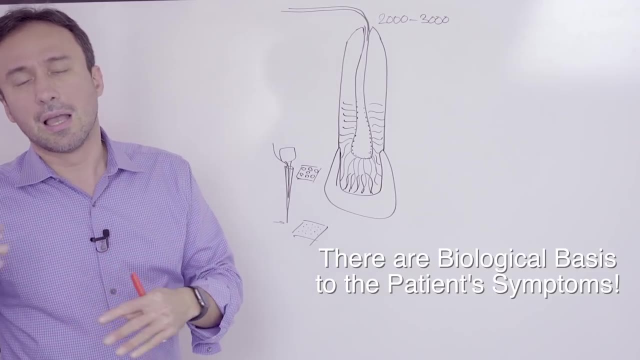 about patients' symptomatology and the way they present themselves as to why is it that some patients have this specific set of symptoms, whereas different stages of disease manifest, for the same patient, a different kind of pain. So we know that all these axons come in. 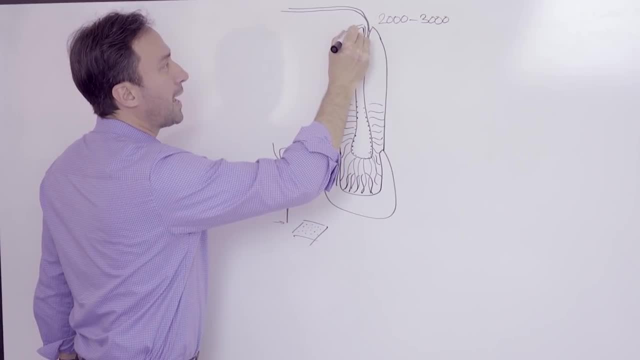 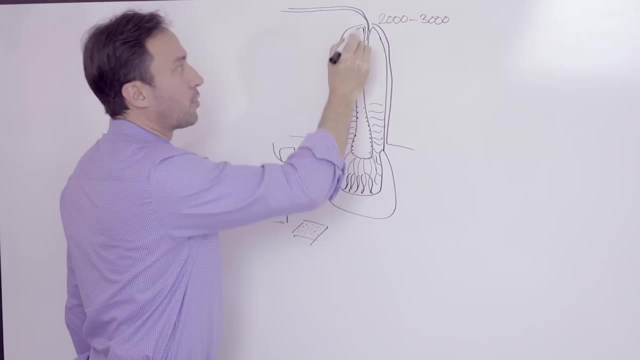 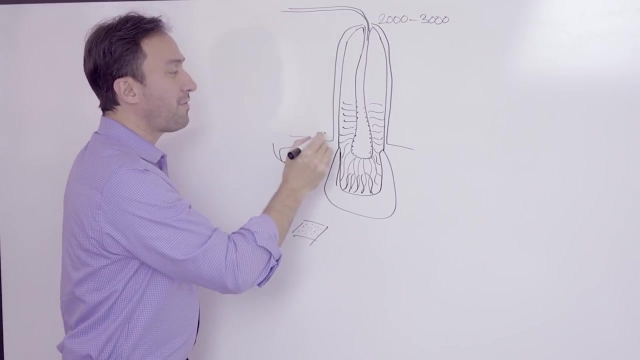 Also, the tooth we know is encased. It's encased in the alveolar socket And the bone. you have some alveolar bone And then the crystal bone that is lining the alveolar socket is in fact cortical bone, which 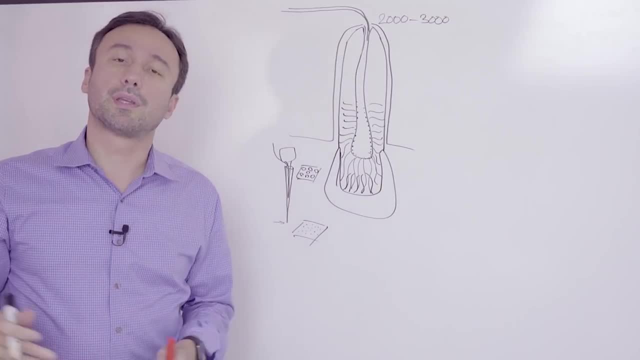 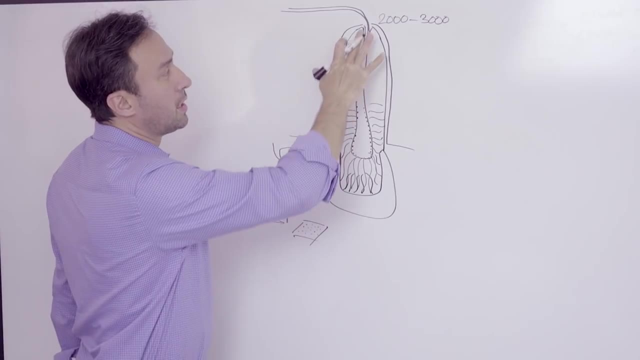 is what, on a radiographic point of view, creates the so-called lamina dura, because cortical bone is what you can see radiographically And that's a significant clinical and radiographic landmark in order to find out how the supporting structures are working out. 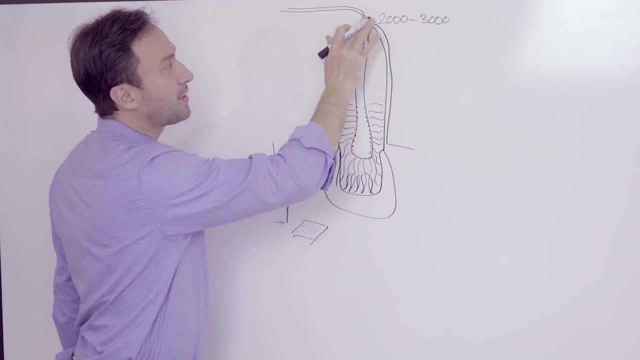 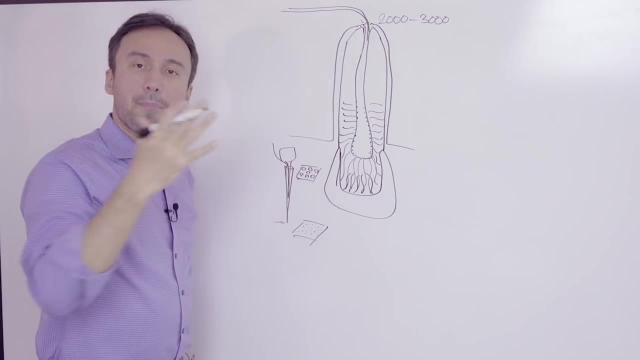 So here, right at the end, you have this area of perforation of the alveolar plate, And that's your cribriform plate, where the neurovascular bundle enters. Now let's get back to the innervation, because it's really, really significant when 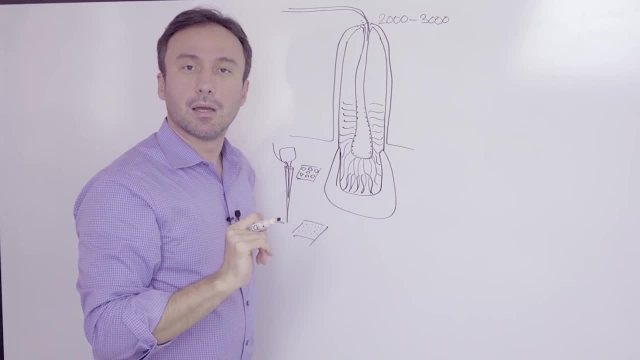 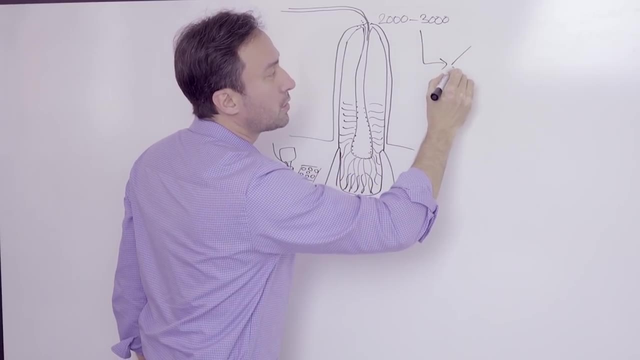 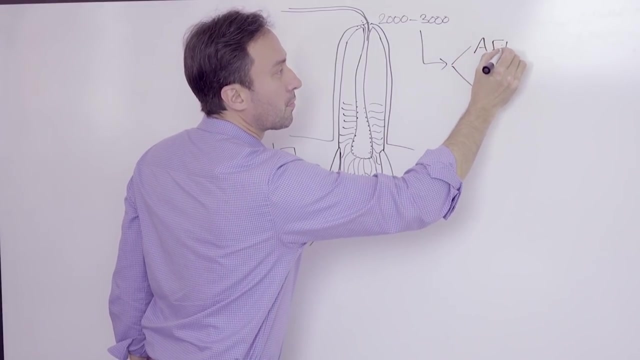 it comes to the pulp, I mentioned that 2,000 to 3,000 axons- individual axons- enter the pulp. These are primarily divided in two different types of nerve fibers: We're talking about The A-fibers and the C-fibers. 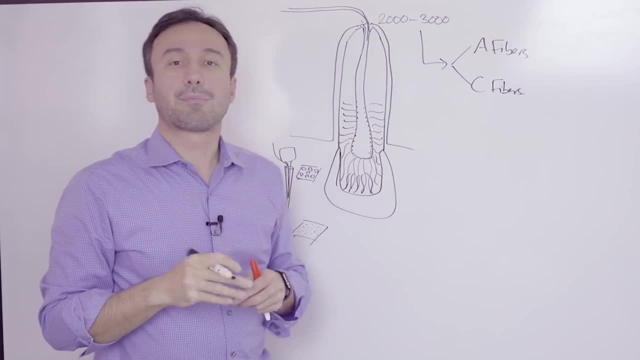 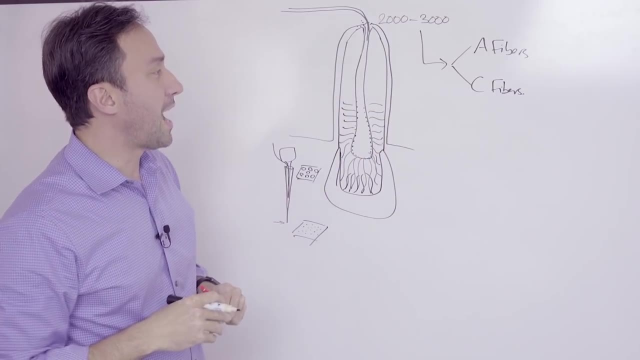 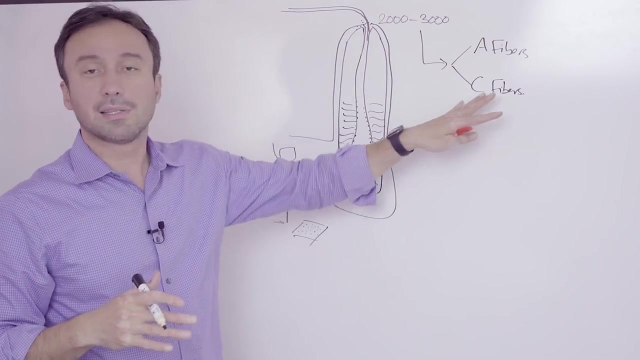 A-fibers are your myelinated, thicker kind of fibers that are responsible for fast conduction of the action potential, And the C-fibers are the thinner, non-myelinated fibers that are responsible specifically for nociception and for slow and dull pain. 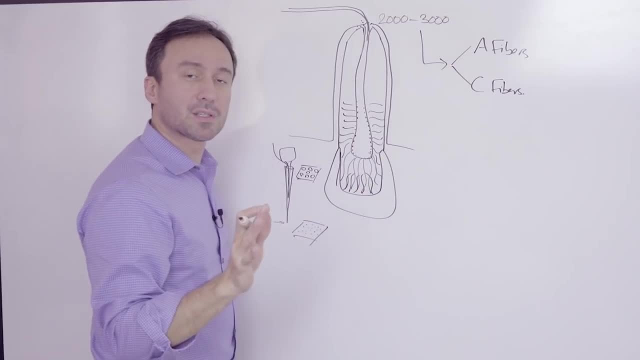 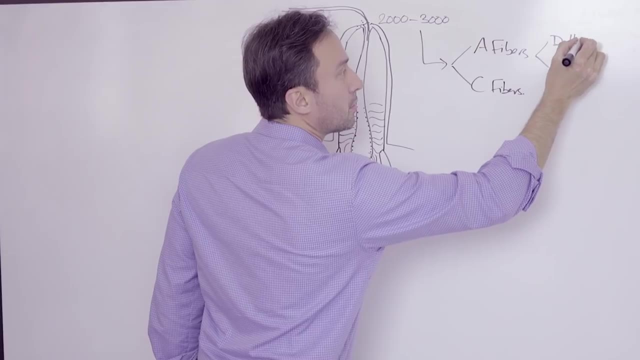 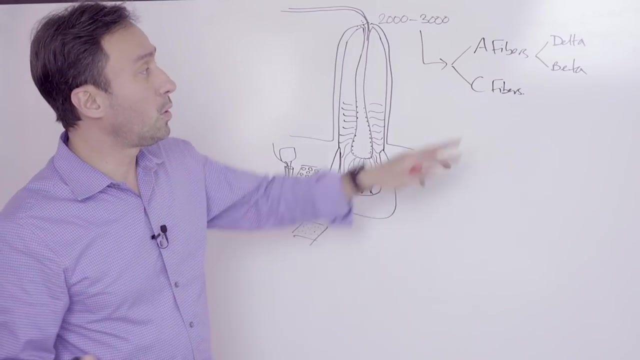 The A-fibers themselves are divided into two subcategories, that are, your A, A-delta and their A-beta fibers. Now, why do you need to know about the A-delta and the A-beta fibers? Well, the A-delta fibers are the most numerous. They account for 90% of the A-fibers in the pulp, And the beta fibers are only 10% of the pulp. So you can see that, OK. Now the A-delta fibers are responsible for the primarily nociceptors. 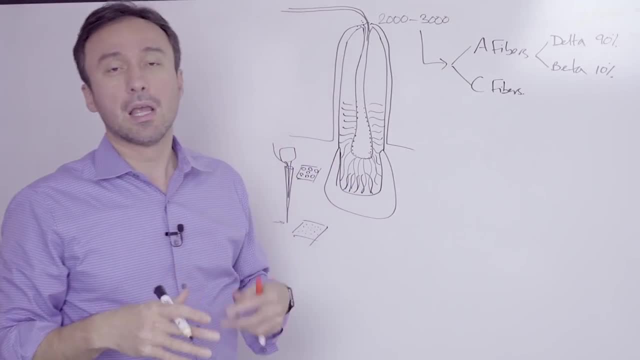 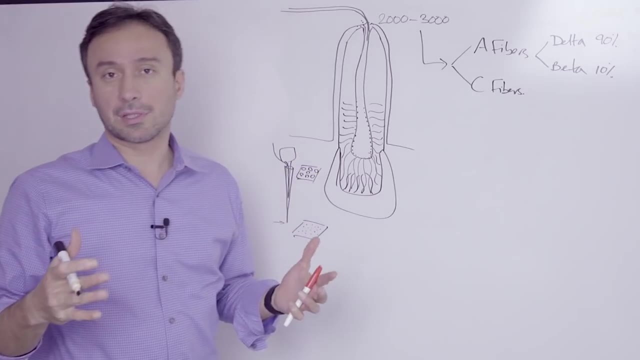 So they create the pain, the sharpshooting pain associated with a toothache. But the A-beta fibers are primarily mechanoreceptors And they're actually proprioceptors. And you can tell right off the bat then, from this kind of a distribution of 90 to 10: 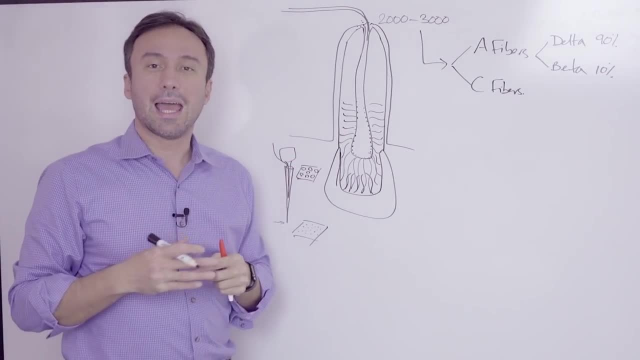 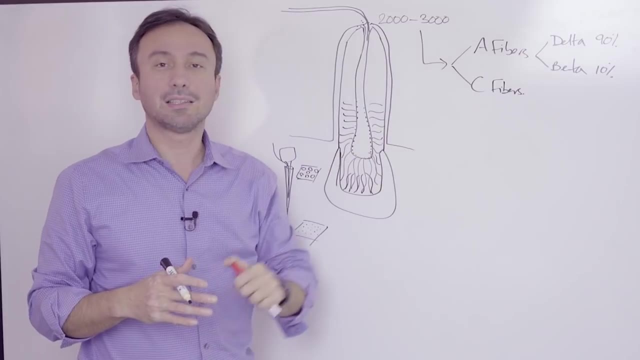 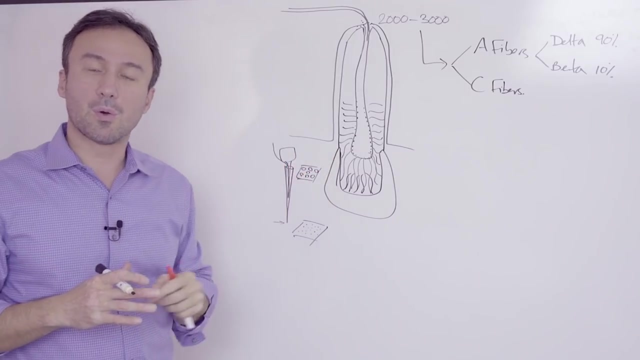 that the dental pulp is primarily a nociceptive kind of an organ. So as a whole, The pain- that is, a combination of the C-fibers and the A-delta fibers that basically leaves the pulp in the afferent pathways and goes up to the brain- is primarily pain. 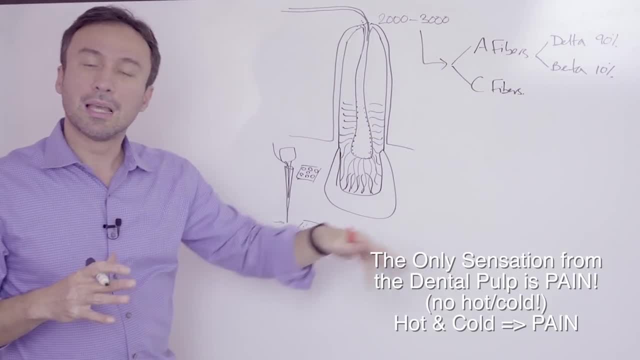 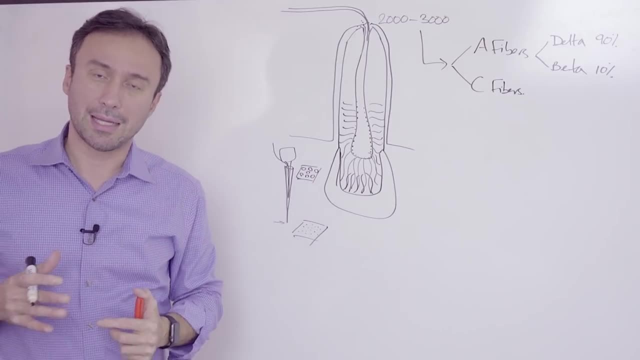 And that the other 10% that is only proprioception. it explains why patients have such a difficult time being able to localize the pain that is stemming from their pulp is because they're really lacking adequate proprioceptive fibers. that allows them to get out OK. 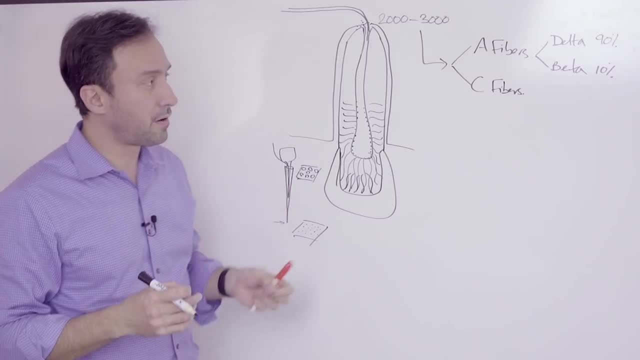 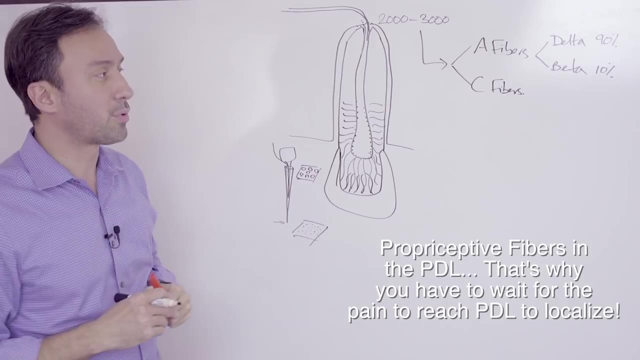 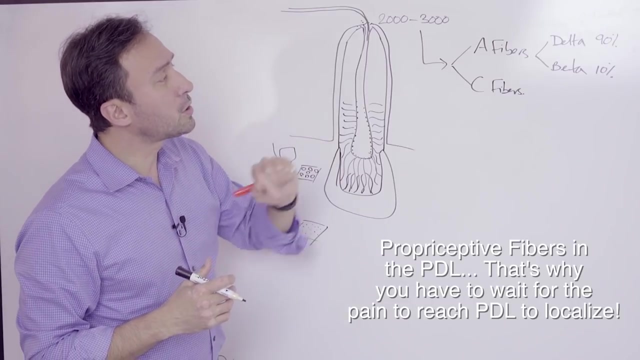 And that allows them to kind of localize the pain. So this is a very significant and important piece of information: that the paucity of these proprioceptive fibers are responsible for our patients being unable to locate their pain. Now, what we need to know is that not only there, 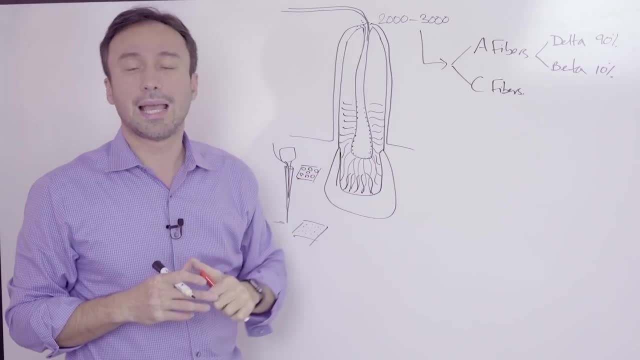 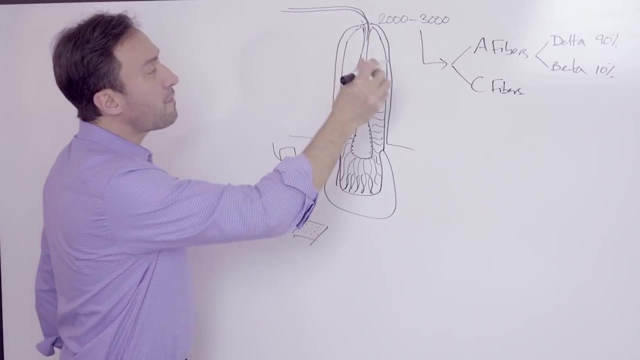 is a difference between the A-fibers and the C-fibers and specifically now with the A-delta and the C-fibers, but there is a difference in the distribution of these nerves in the dental pulp, The A-fibers primarily when they enter here from the end. 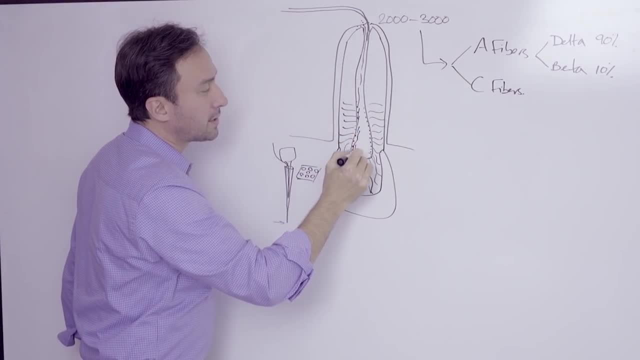 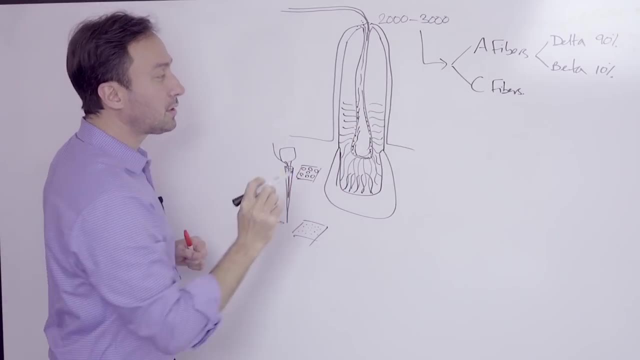 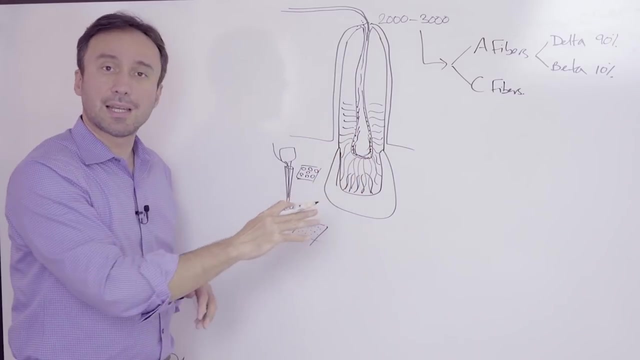 they end up creating a plexus, so-called the plexus of Raschkow, which lines the periphery of the pulp. These are the A-delta fibers, are the ones that create this dense plexus of nerves right adjacent to the dentin. 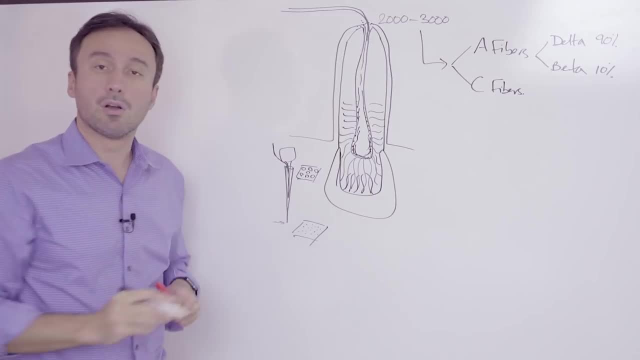 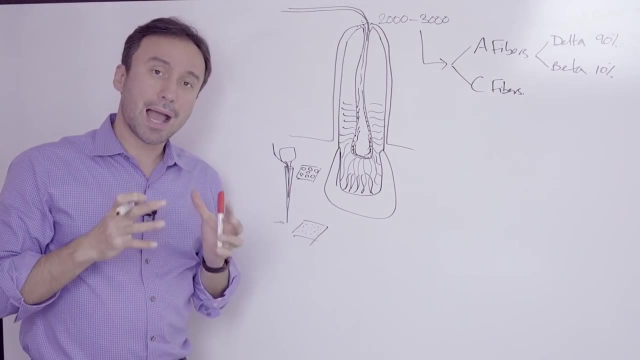 And these are the guys responsible for sending individual axons into the dental tubules. So, therefore, because they are A-delta fibers, that are, myelinated fibers, that explains why the pain that you get from dentin is a sharp shooting one. 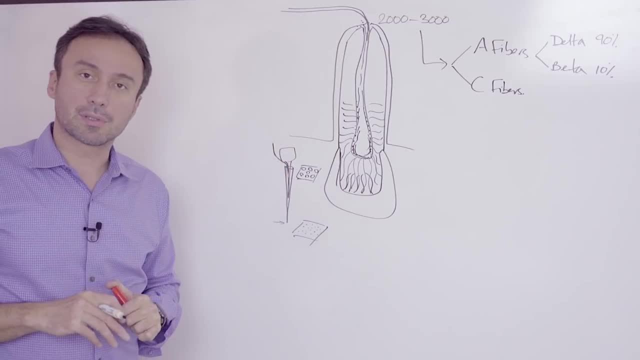 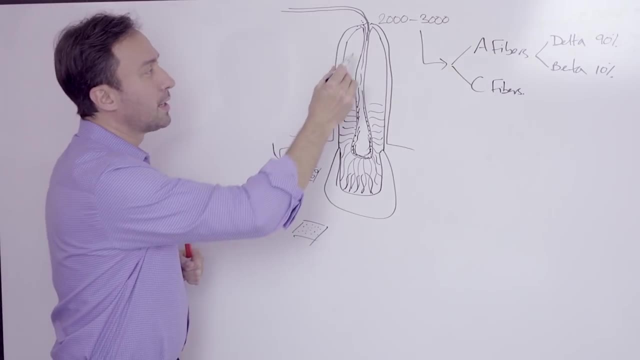 because that's the kind of pain that the A-delta nociceptors tend to kind of conduct. The C-fibers, on the other hand, that are the unmyelinated thinner ones. they kind of stay right in the middle of the pulp. 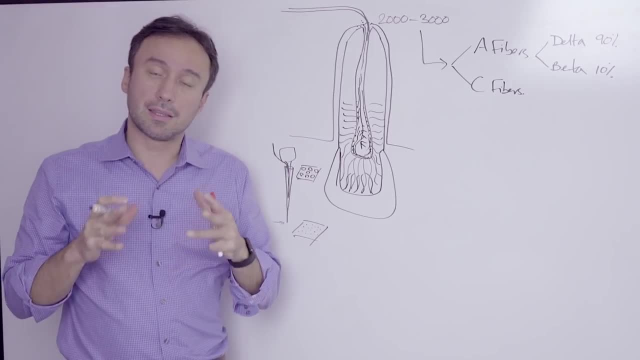 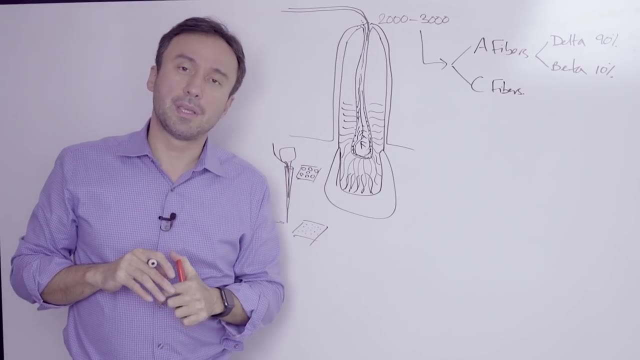 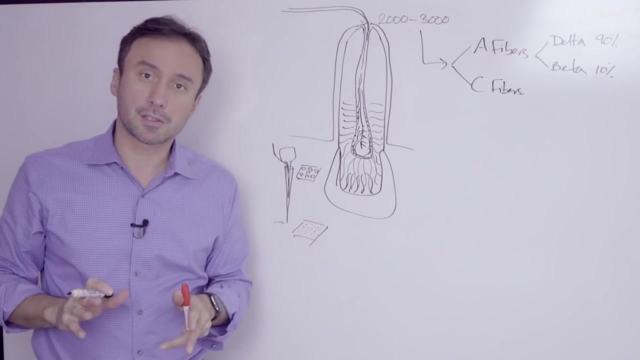 and they branch out, And these are the. they stay in the center of the pulp, in the so-called pulp proper. So that gives us another piece of information here to understand. What it means is that the peripheral area that gets inflamed first is giving us the sharp shooting pain. 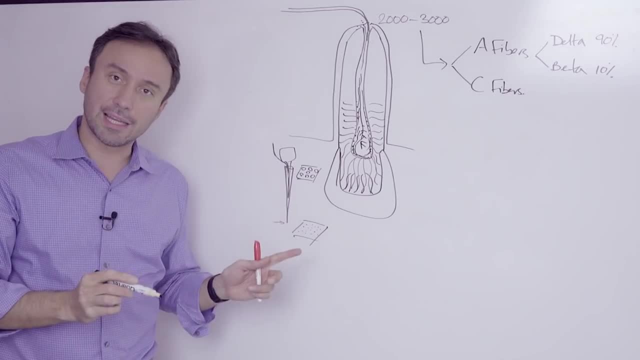 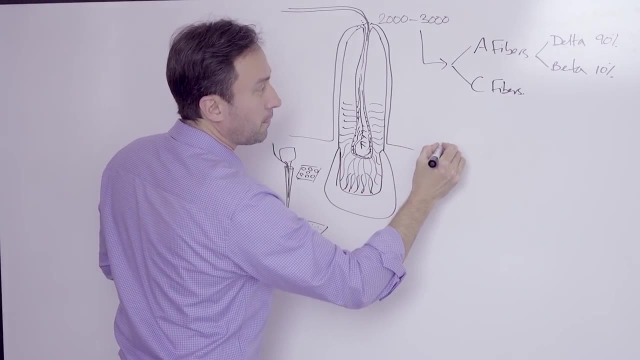 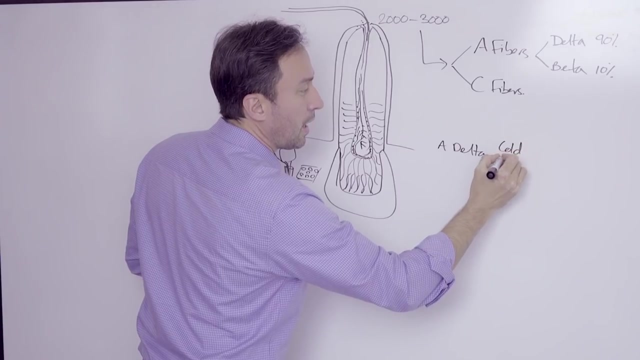 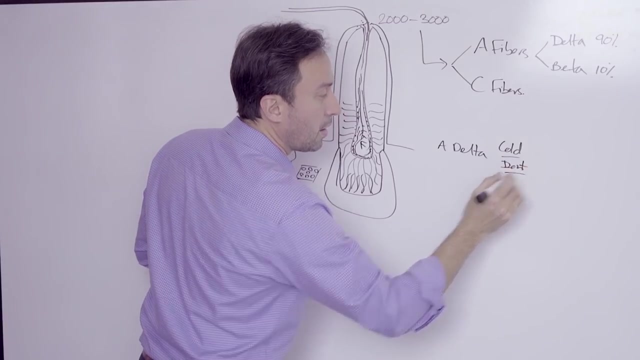 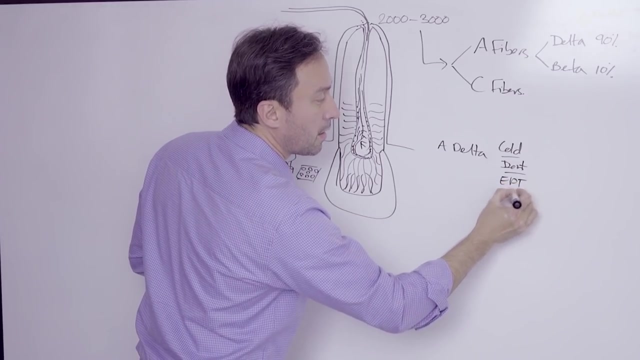 And because the mechanism is dentinal sensitivity, cold sensitivity is triggered by the A-delta, So A-delta fibers give us cold sensitivity and also the dentinal sensitivity right. Also, it's important to note that these are the same fibers responsible for doing our EPT testing. 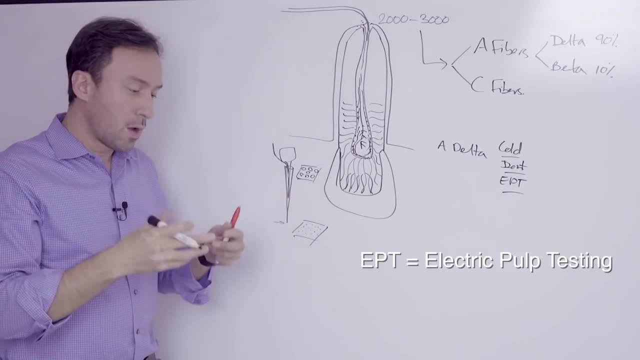 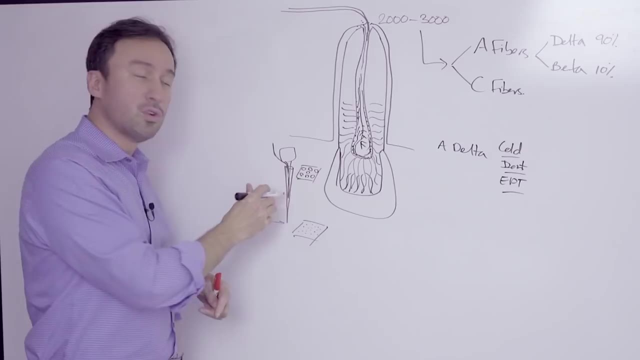 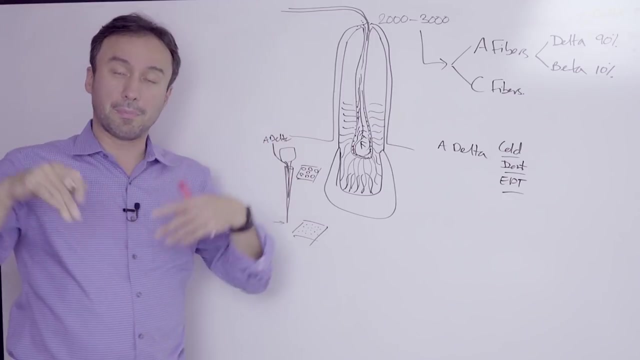 When we do our cold testing, when we place cold on a tooth, what the cold does is it causes contraction of the intratubular fluid And this contraction creates fast movement, which triggers the A-delta fibers, And these A-delta fibers give us a sharp shooting pain. 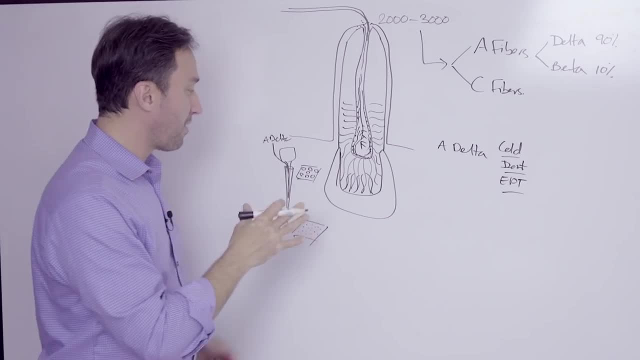 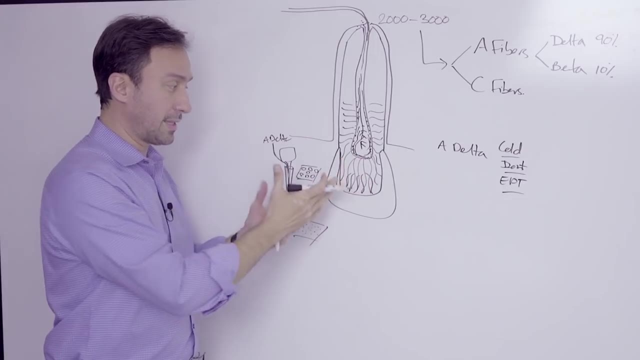 that goes up to the brain And the patient will certainly respond about that Later on. so, as you can see, the peripheral nerves will die first because they're closest to the dentin, And that's the injury, or the caries starts from outside. 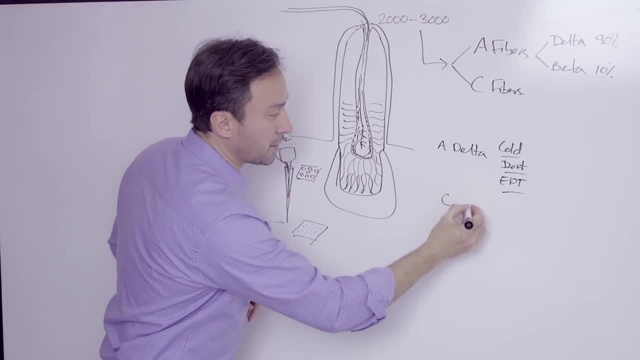 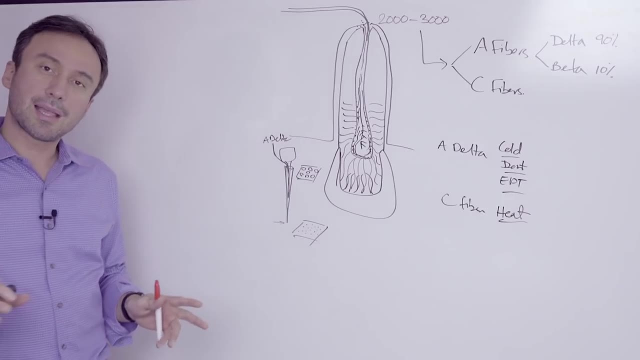 and moves to the middle The C-fibers. on the other hand, they're responsible for your heat sensitivity. So now it's starting to make sense, right, Because you always? poplitis in general starts from some kind of cold sensitivity. 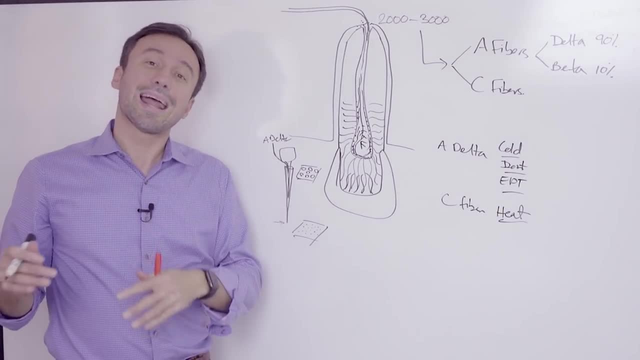 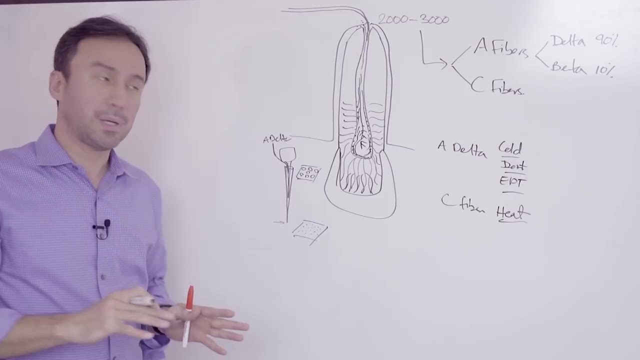 And then in later parts of the disease it moves on to heat sensitivity. And this is the mechanism for why that happens. The reason is because first the A-delta fibers that are in the periphery get involved. The patient recognizes those symptoms. 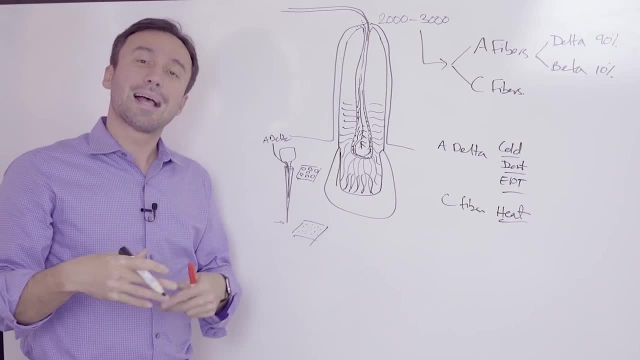 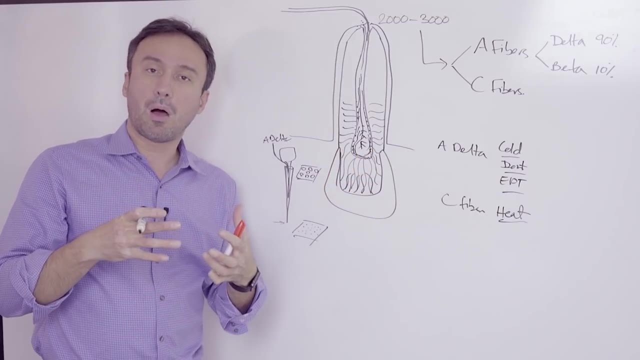 And then they move on to heat sensitivity. And then they move on to heat sensitivity As the pathology progresses and inflammation starts to spread deeper into the tissues and ends up in the pulp proper. now your C-fibers end up getting involved And they're responsible for your heat sensitivity. 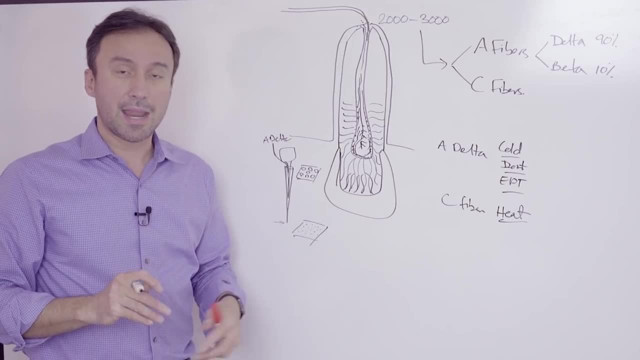 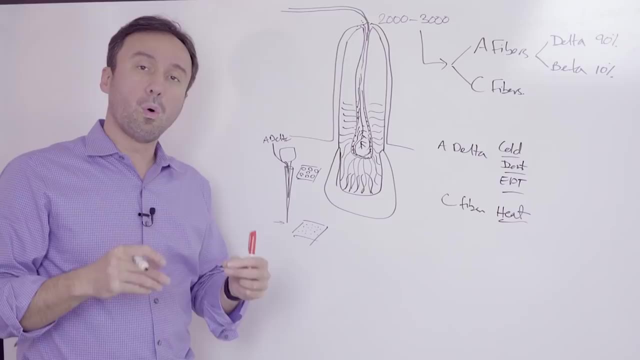 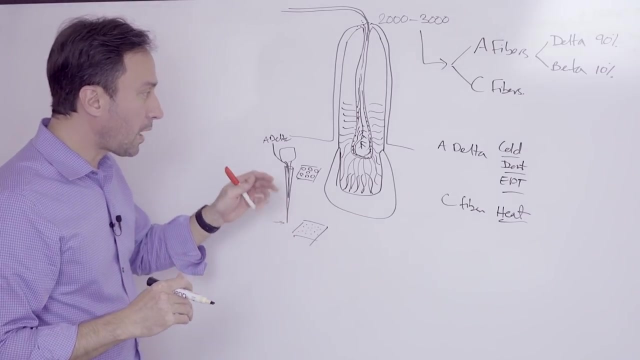 So patients later on end up having heat sensitivity. Now we also- all of us- have seen clinically patients who come in with severe heat sensitivity where only cold will help alleviate the symptoms. And what that is? it is essentially a situation in which heat causes vasodilation. 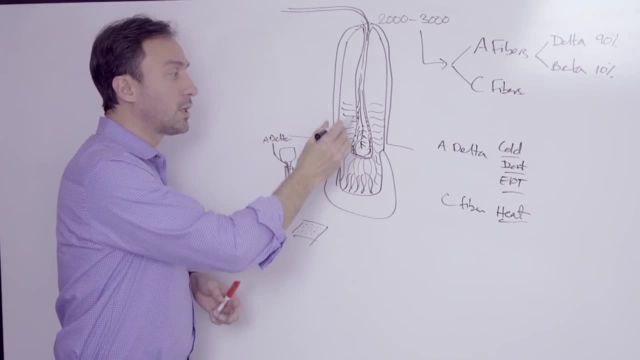 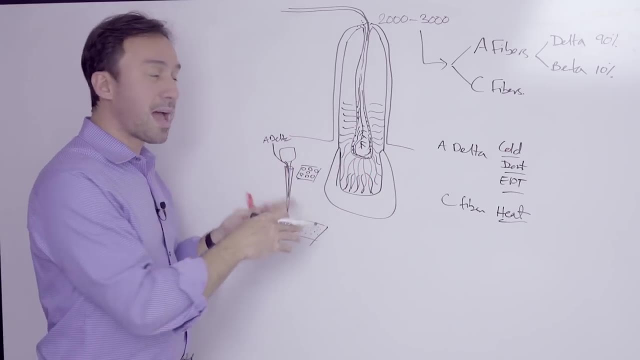 And what the vasodilation does at that stage is it actually creates, it increases the pulpal, intra-pulpal pressure And that triggers the C-fibers. But then, at that point, once the C-fibers are dead, 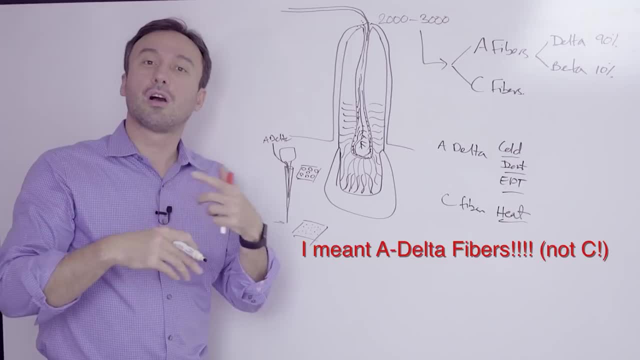 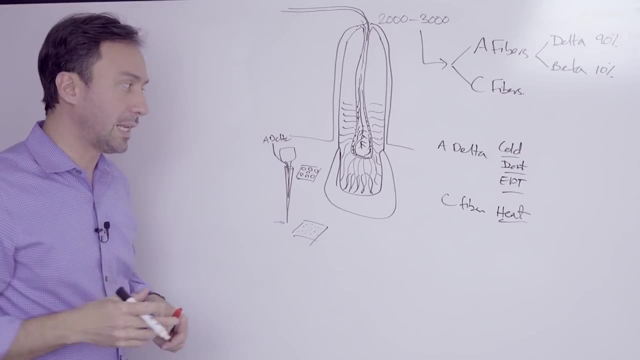 because they're the periphery, the cold will actually cause vasoconstriction, which will alleviate the symptoms from the heat which is triggered, as I mentioned, by vasodilation, vasodilation, vasodilation, vasodilation. 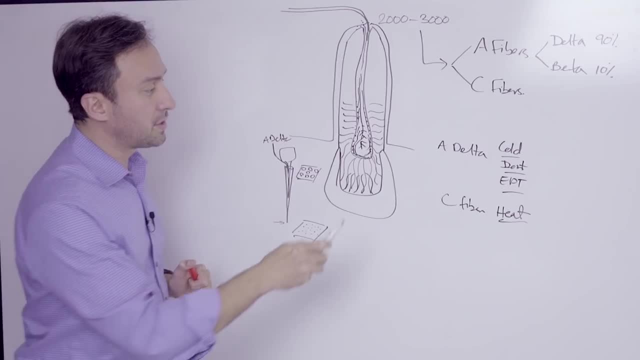 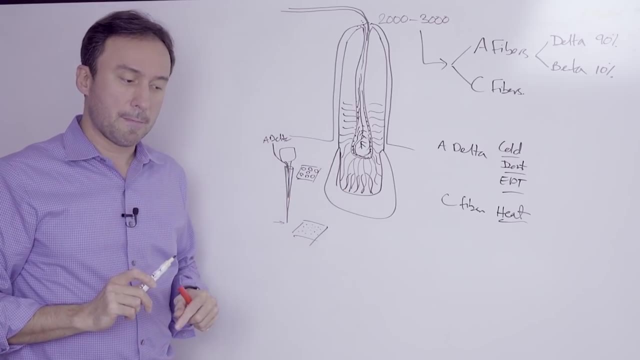 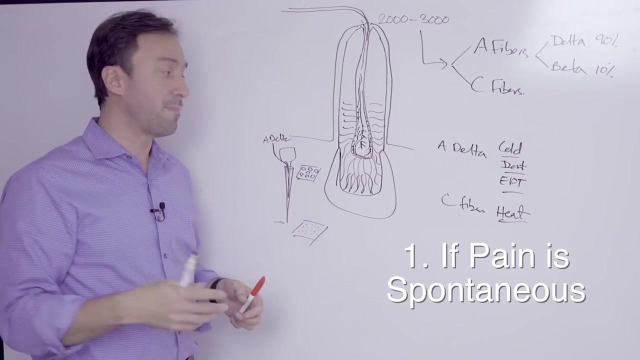 vasodilation. It's an important concept to understand as well. This is how the progression of the symptoms go on. We all know that our inflammation ends up being irreversible through two criteria: If the pain becomes spontaneous and that means that the inflammation has become more widespread. 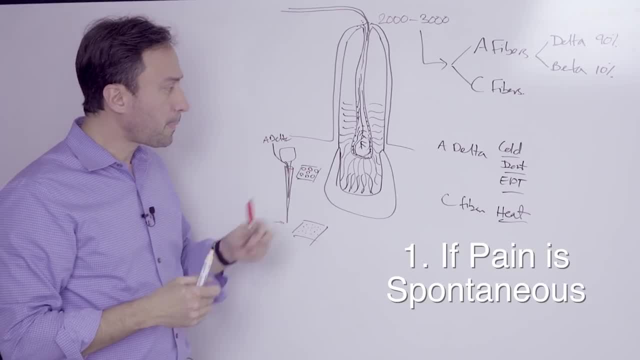 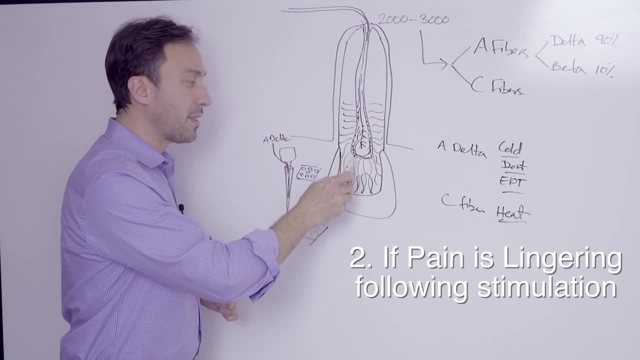 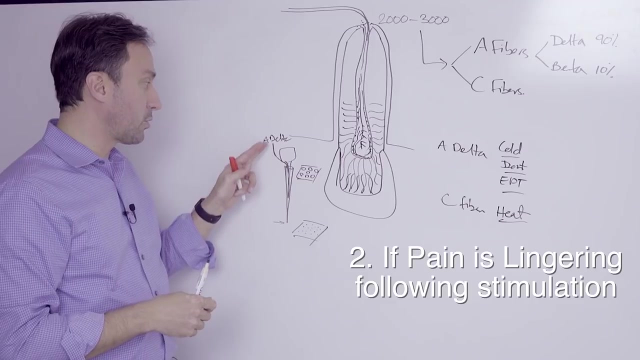 and is more in the pulproper, And also if the response to thermal stimulus becomes lingering, In which case that means that it isn't just a mere contraction of the fluid. It is beyond the contraction of the fluid that's triggering the A-delta fiber. 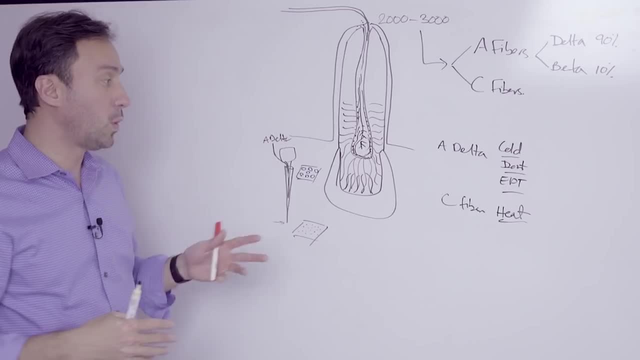 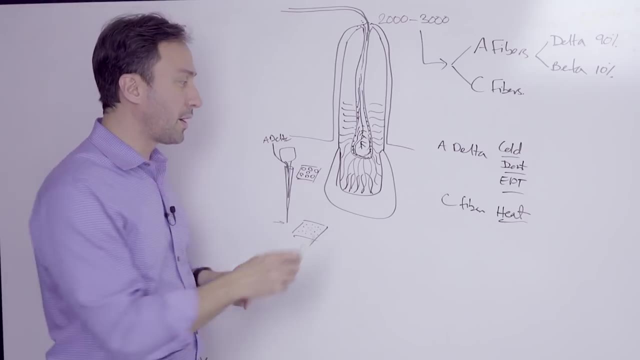 It's actually due to physical injury to the pulp as well as the pulp proper. So these are important things to understand. So we learned several important concepts. We learned about the concept of permeability of dentin, which is very significant for all your restorations. 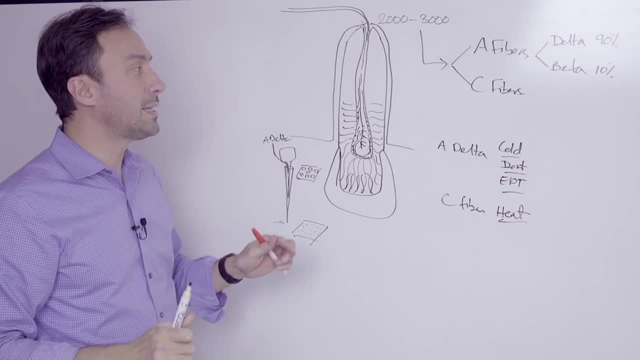 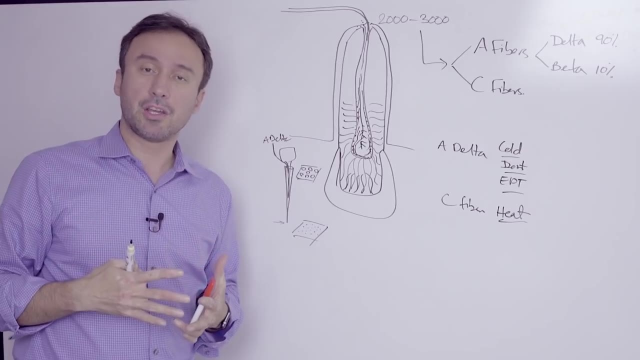 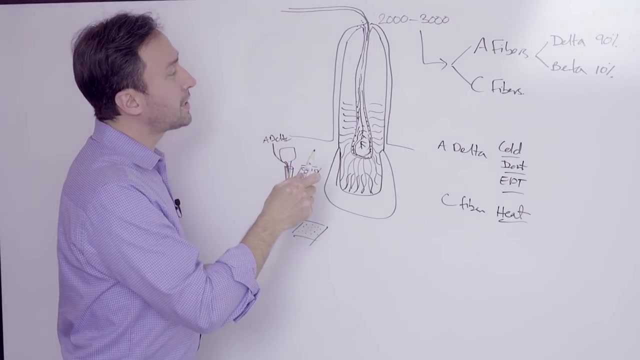 We learned about the innervation of the pulp And how it signifies different pathognomonic symptoms along the cascade of inflammation in the patient that is reporting to you with a chief complaint of pain. But now let's take a look at also. 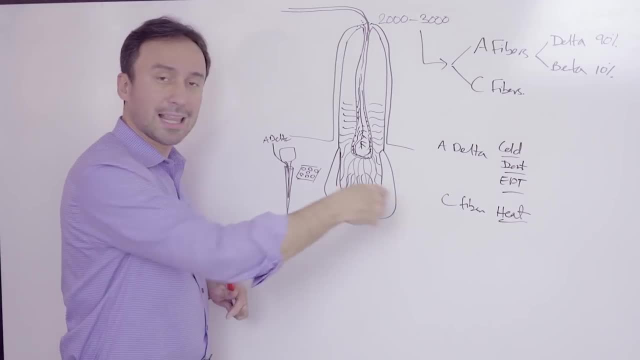 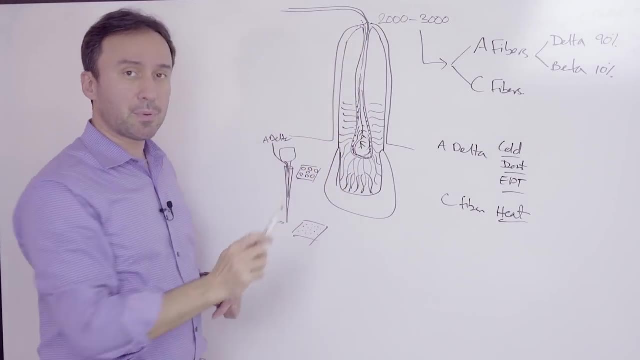 this is inflammation in the pulp. At this stage you have to do a vitality test and so on to find out about the condition. Once this inflammation inside the pulp progresses and moves down to the apical area, then you end up getting inflammation. 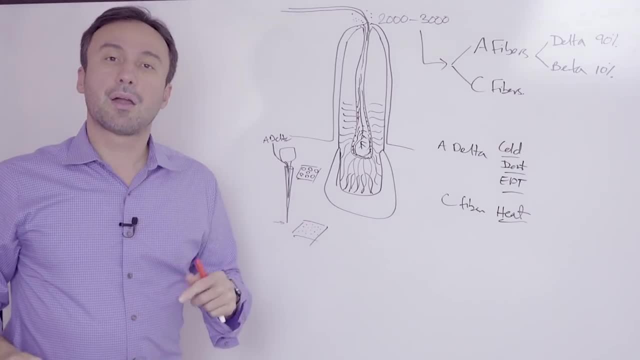 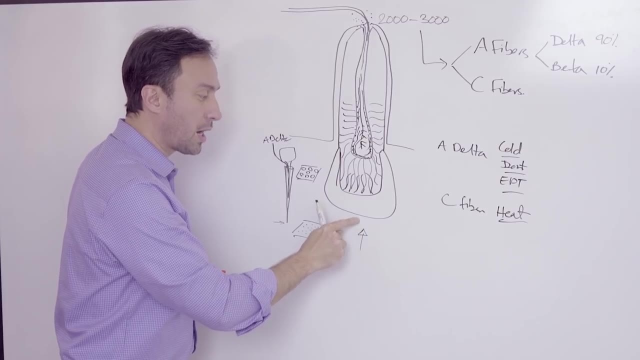 down to the pulprical area Down here, And when you get inflammation down at the periapical area, that's when your percussion test become valid, Because at that point when you percuss on the tooth, the whole tooth and the root becomes. 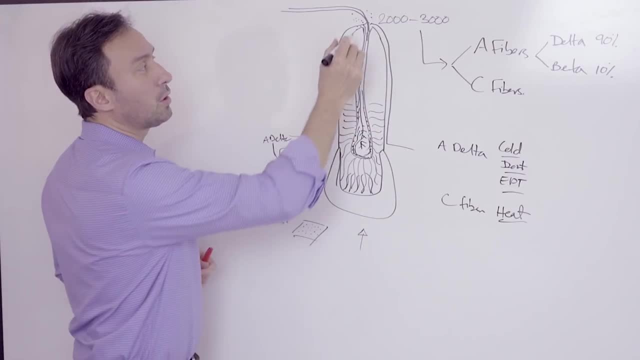 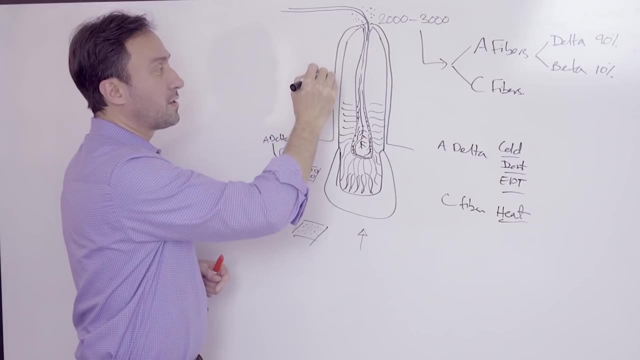 an extension of your mirror And basically all you're testing at that point with your percussion test is the status of the periapics. Of course, it also gives us information about the lateral areas of the tooth, whether there is inflammation there. 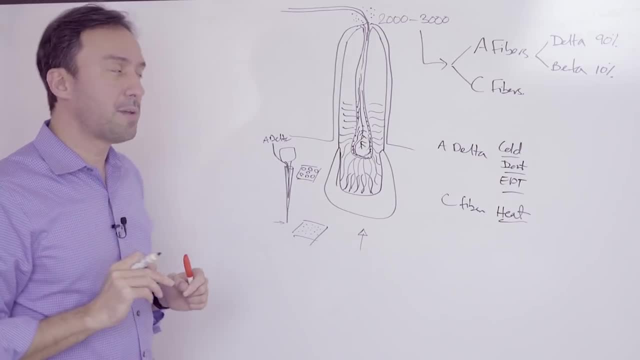 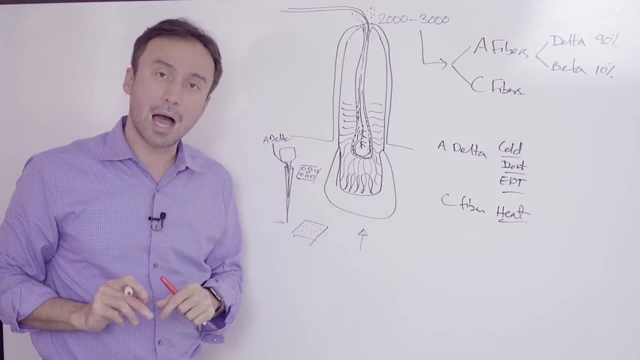 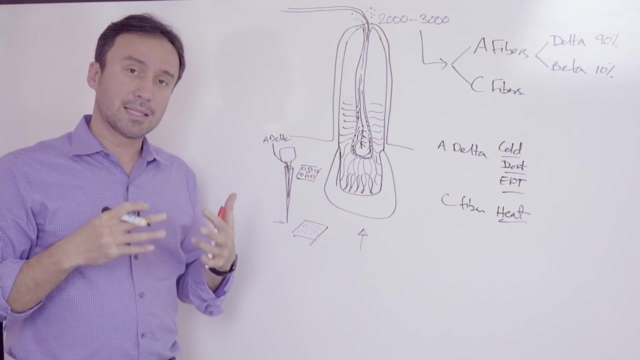 So it's not only right at the apex, But let's see. why is it that the pulp actually dies? The reason why the pulp dies in cases of inflammation is because, as I mentioned, it's an encased area. Now it is encased. 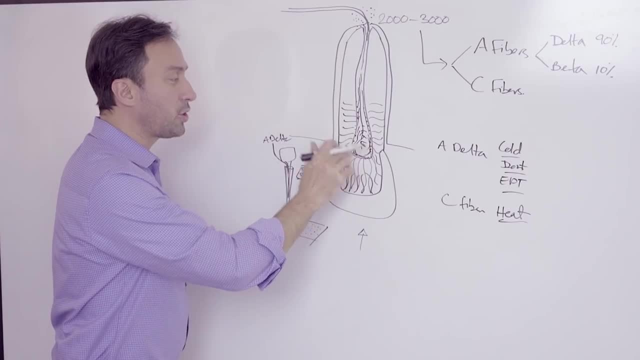 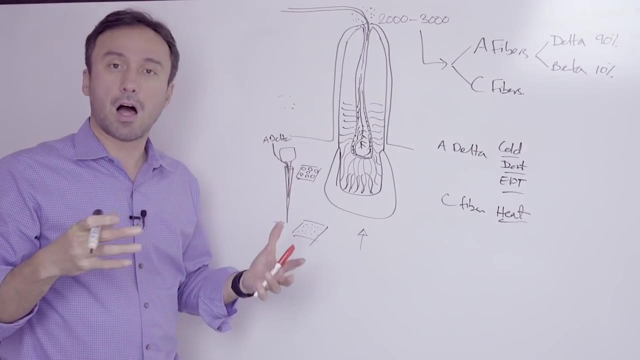 And as a result of that, the same amount of inflammation, just like out here in the bone or in the soft tissue, would allow an increase in the volume, And this increase in the volume would be as a result of the inflammatory exudate. 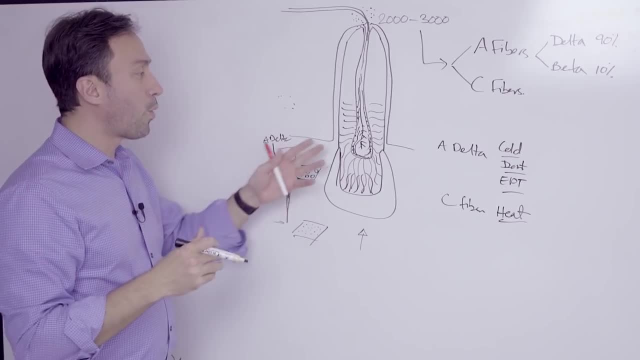 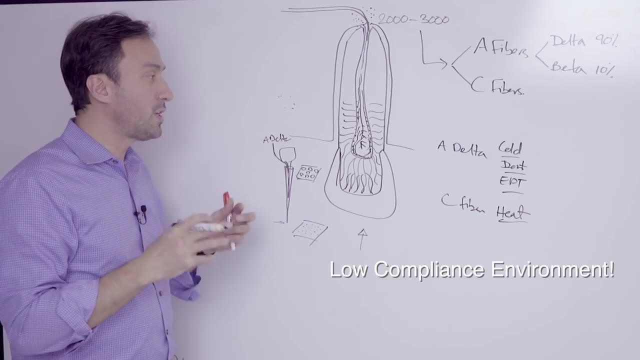 that comes to the area to fight the source of the injury. However, in the pulp, because it's encased, there is no chance for an increase in volume, And the increase in volume actually translates into an increase in intrapulpal pressure. 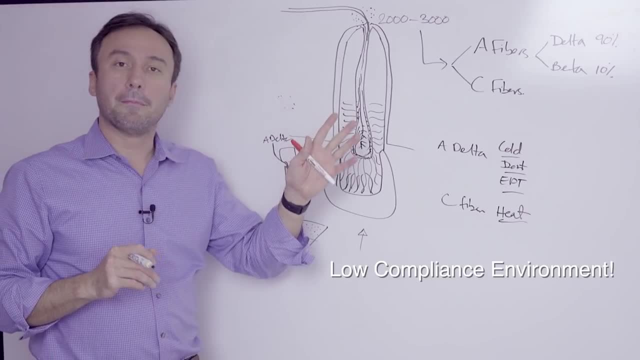 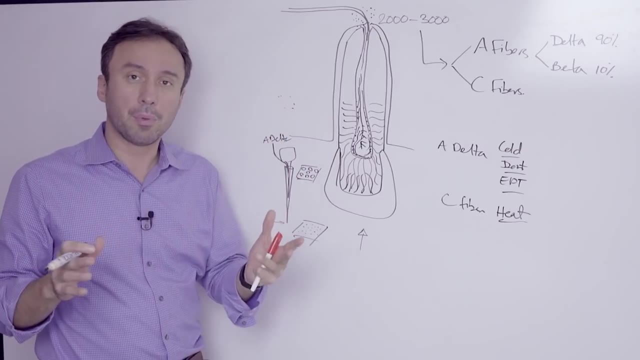 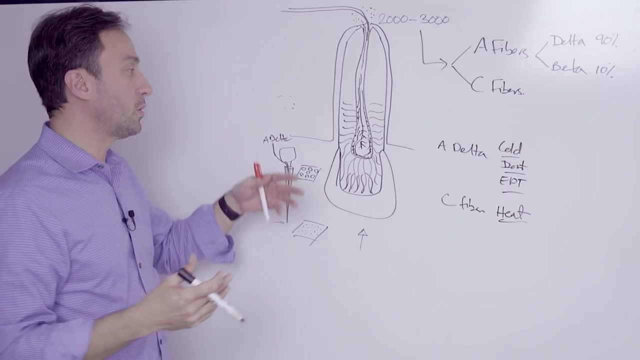 And an increase in intrapulpal pressure basically ruins the entire circulation system, And because we don't have the so-called collateral circulation in the dental pulp, what ends up happening is that you end up going through a necrosis rather than a typical situation, which would mean inflammation. 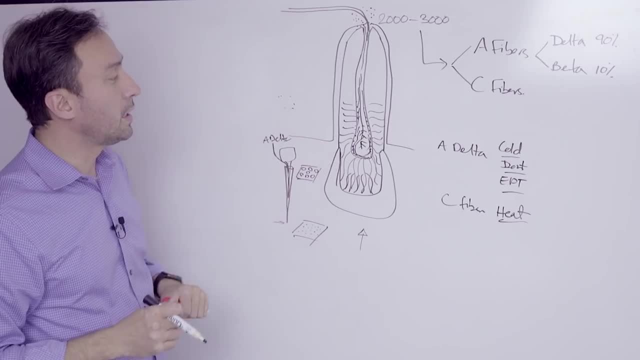 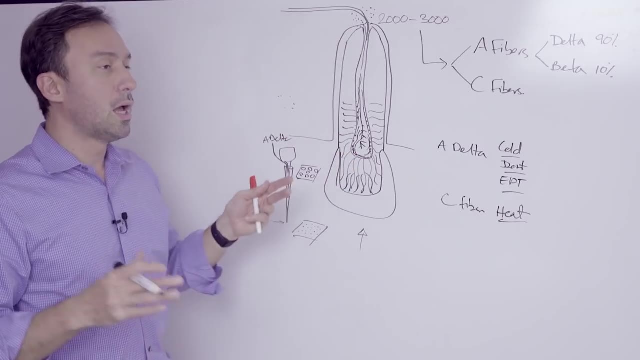 followed by repair and regeneration. In the case of the pulp, you end up getting necrosis And the necrosis results into an empty space that could then be infiltrated with bacteria chronically and then end up shooting out the end of the root, which 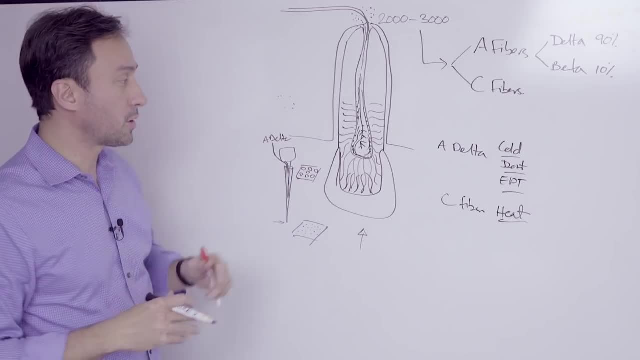 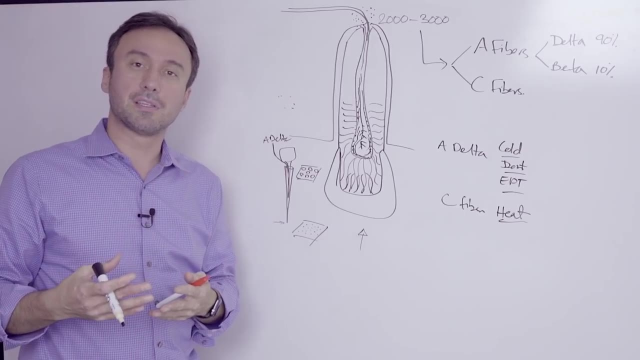 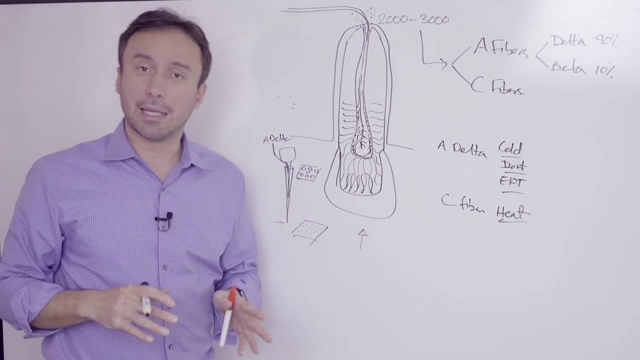 will then maintain the infection, hopefully, of course, the entire essence of root canal therapy is to understand the physiological basis of this process and then get access to this space, which has now become a dead space, decontaminated, disinfected, remove the bacterial source. 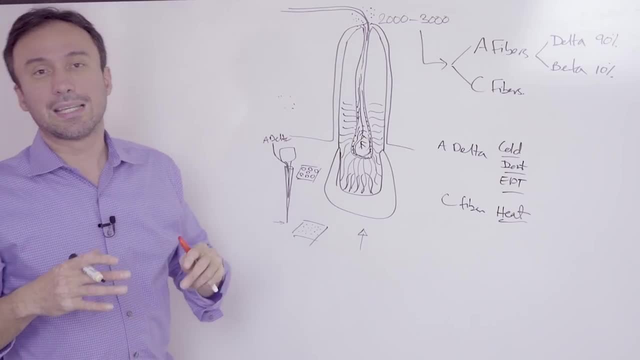 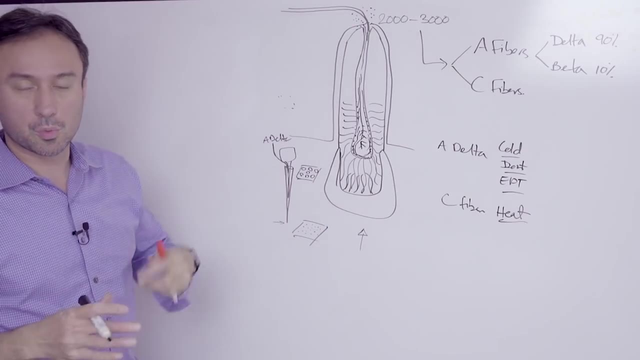 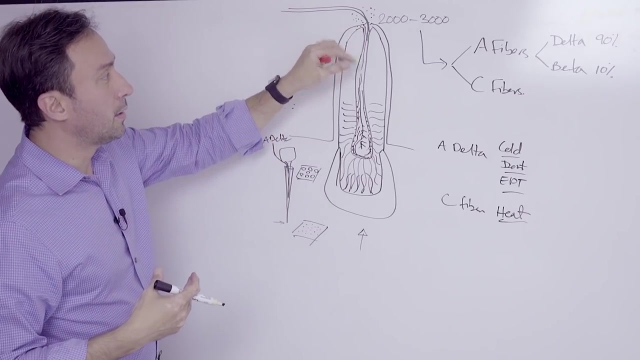 and the burden and then obturated, which would then eliminate the space as a potential source for egress of bacteria into the periapical tissues, which will then maintain the infection Once we remove this source, which is removing the source of the injury to the periapical area. 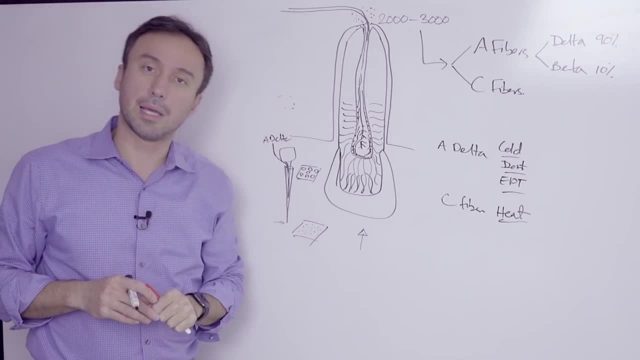 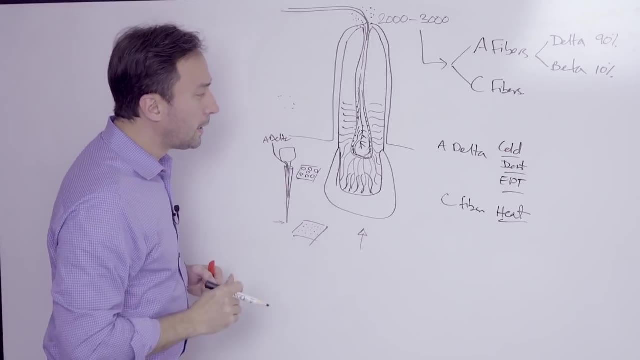 the area outside would heal no different than any other place, And that is basically the essence of the root canal therapy and the root canal story, if you will. But let's just go back and talk a little bit about some of the other symptoms that 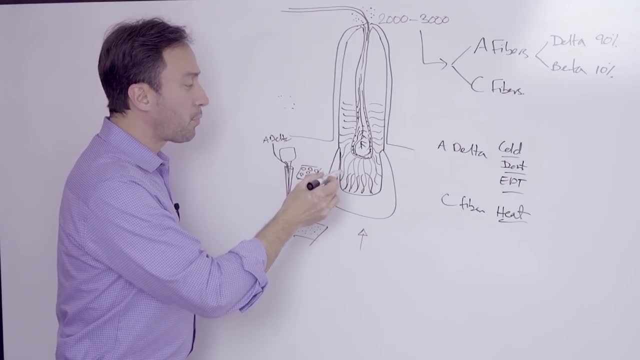 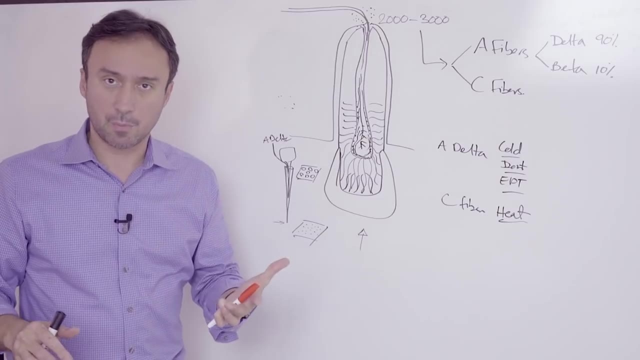 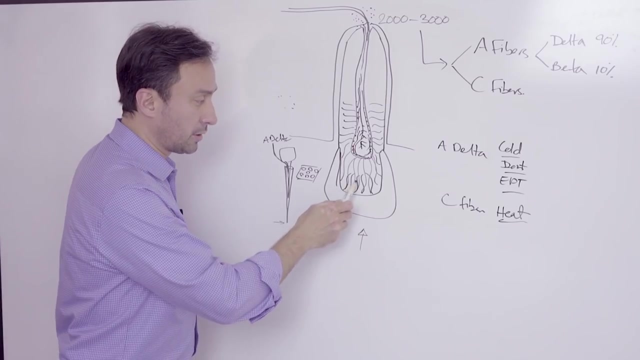 occur clinically in patients. For example, what is the problem when you end up having the difference between a percussion response versus a biting response? What ends up happening is when you're having a patient bite into a tooth's fluid, you end up having cuspal deflection. 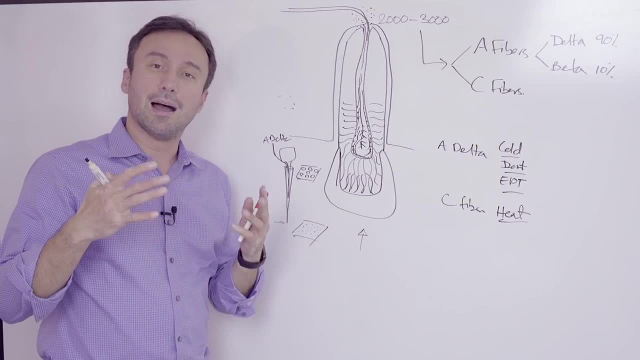 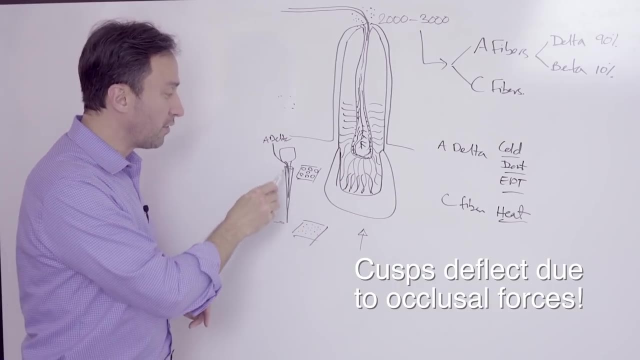 And what this means is that the tooth is not quite as rigid as we may think. There is movement, And this movement always translates into the same issue of movement of the fluid into the dental tubules, which is why, if you either have a crack, And the tooth which will allow this opening and closing of the crack, which increases the fluid movement and creates a sharp pain. Or if you have a restoration but your restoration doesn't have a good bond, If you've lost the bond on your restoration. 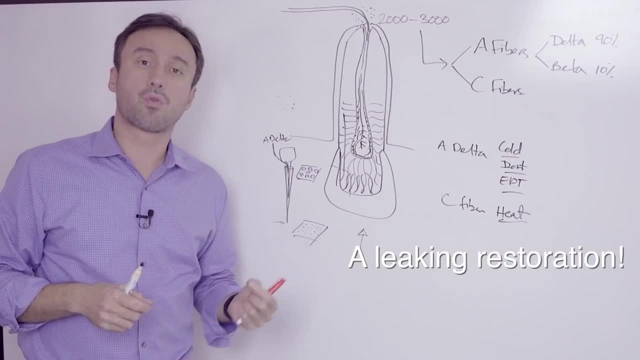 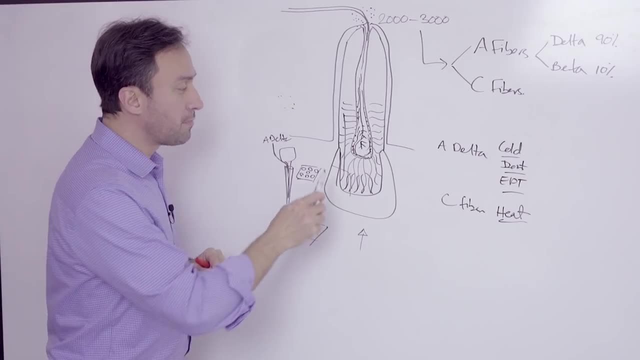 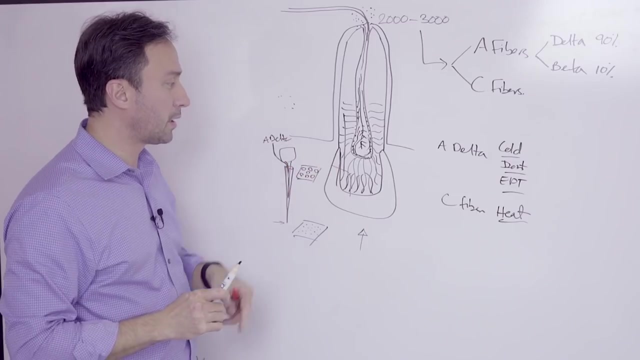 your restoration will basically give you the same response as a crack would, because the margin ends up acting like a crack. So you have to keep that in mind, that all of the sharp, zinging or fast action, that all of the sharp, zinging or fast action. 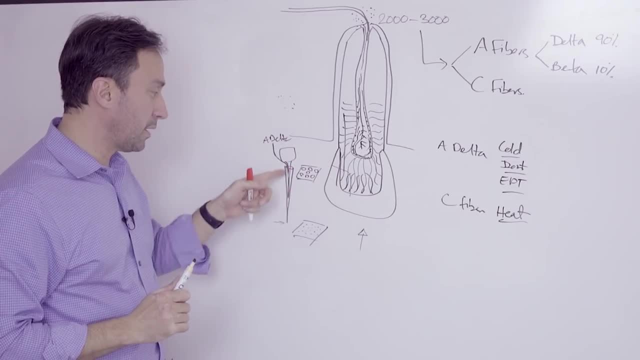 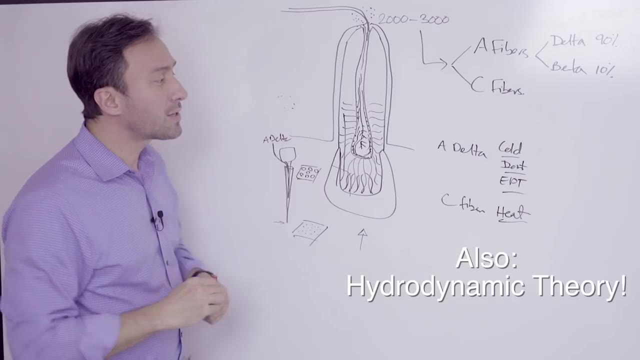 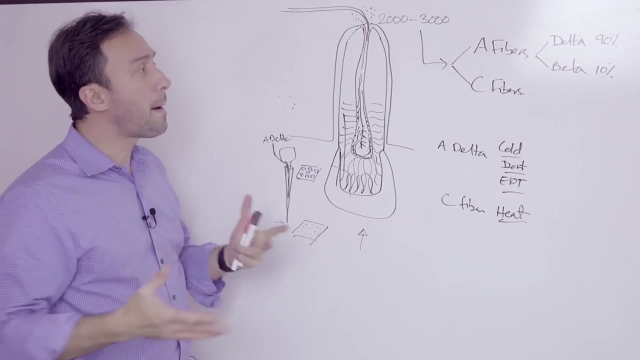 is a function of fluid movement in the dental tubules, which is actually called the Brandstrom theory of dentin hypersensitivity. Anyway, so these are some of the underlying bases of pulp biology and I think everybody should be aware of And I think we're going to come back to these in the future. 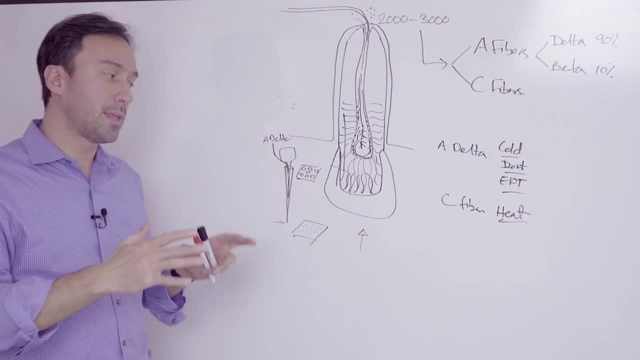 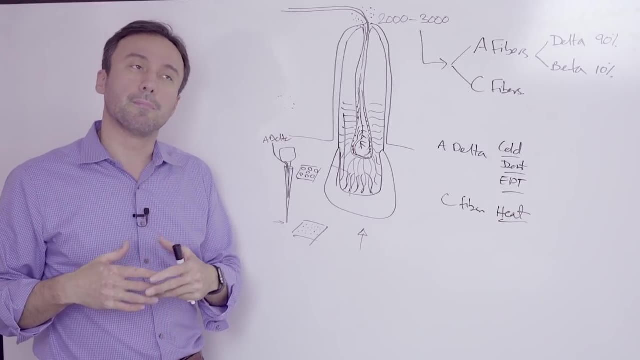 And their significance should be the underlying theory or the scientific basis upon which we build the theory of dentin hypersensitivity, And I think we're going to come back to these in the future. And I think we're going to come back to these in the future. 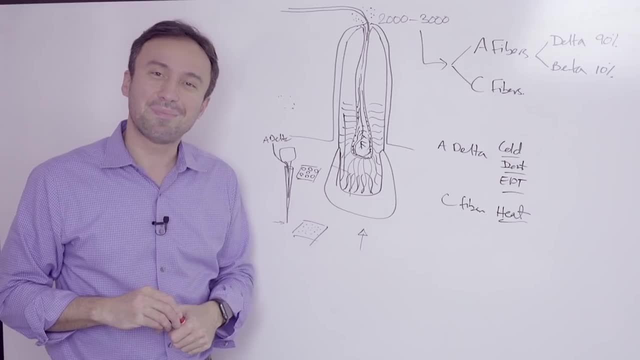 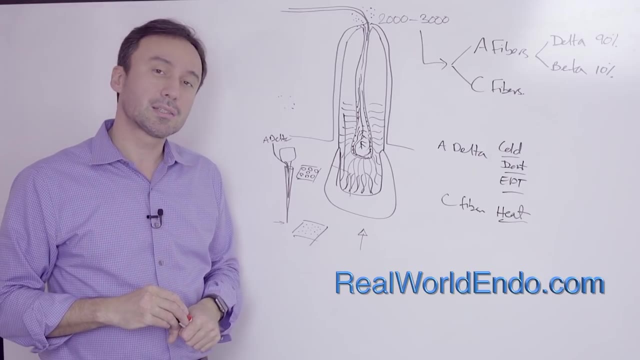 Anyway, I hope this was informational to you and I hope nobody fell asleep during this. But if you have any questions, don't forget to post them in the Ask the Faculty Questions section of our website at rewoldendocom. And for rewoldendo, I'm Ali Nesse. 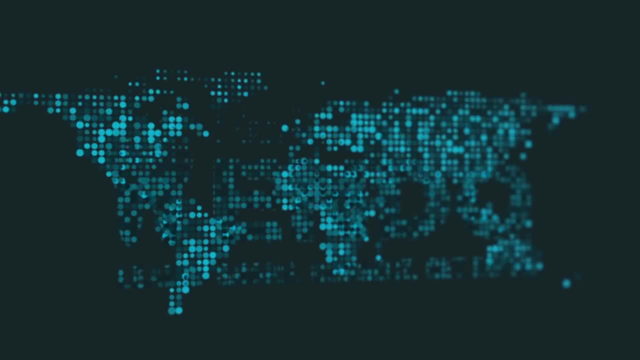 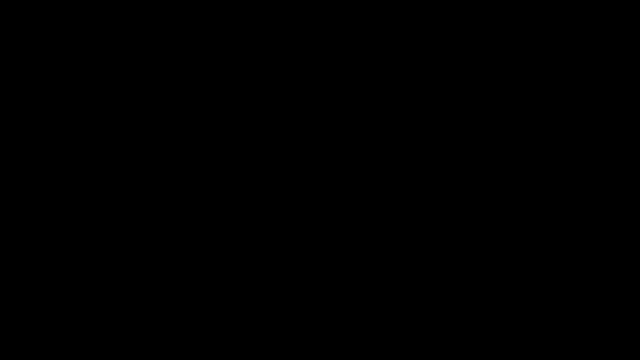 and I hope you found this information helpful And I'll see you in the next one. 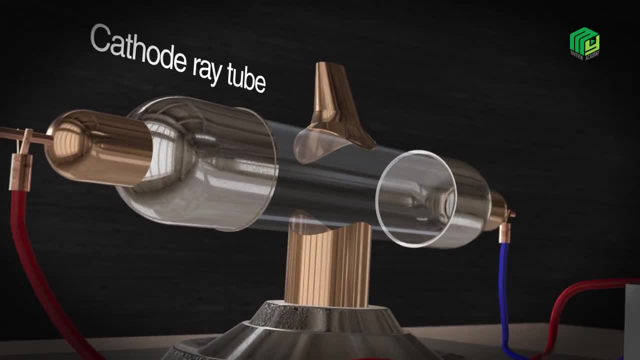 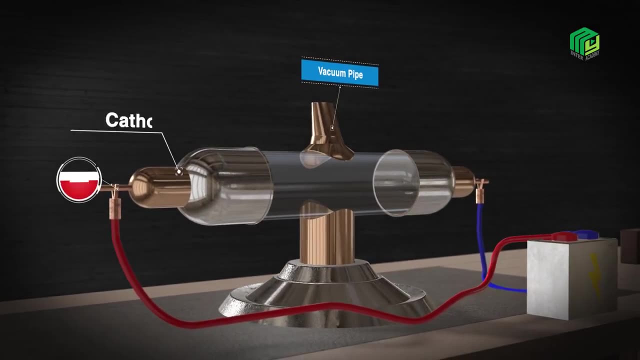 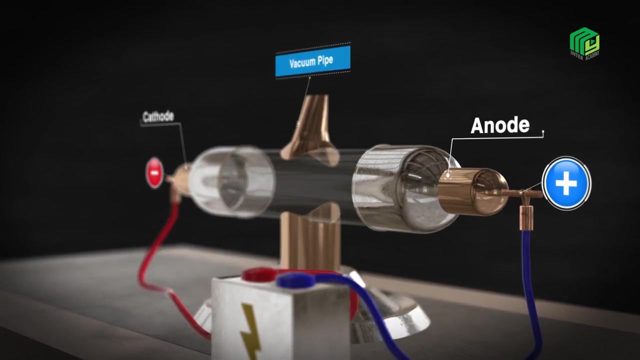 Cathode rays are produced in a discharge tube. A vacuum pump is used to evacuate the discharge tube. The cathode of the tube is connected to the negative terminal of the battery and the anode of the tube is connected to the positive terminal of the battery. It was observed. 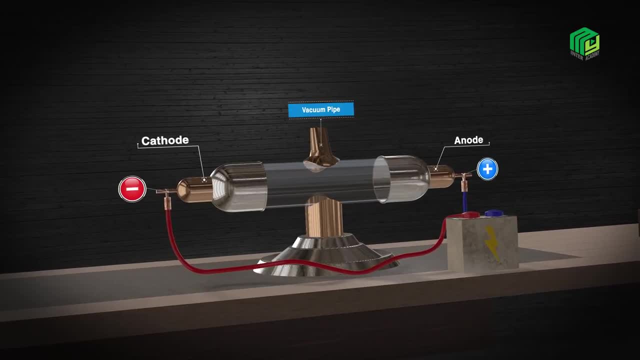 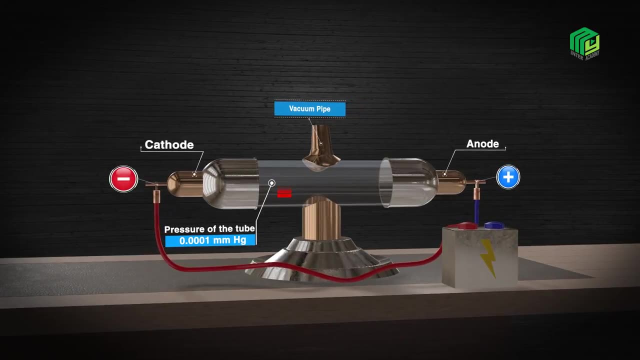 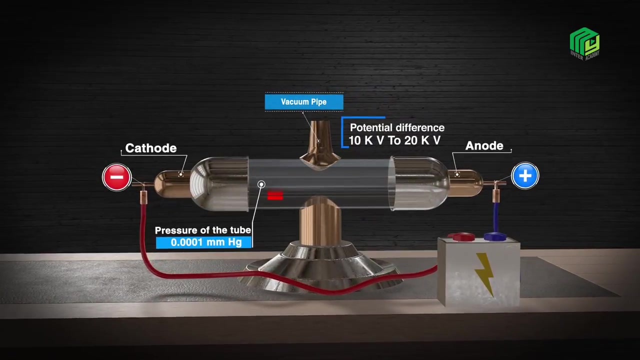 that at normal pressure, the gas did not allow the current to pass through it. However, when the pressure of the tube was reduced to 0.001 mm Hg and a high potential difference between 10 kV and 20 kV was applied at the end of the tube, a glow was seen on the walls. 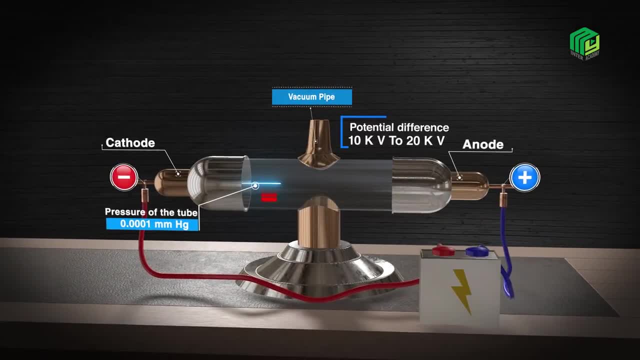 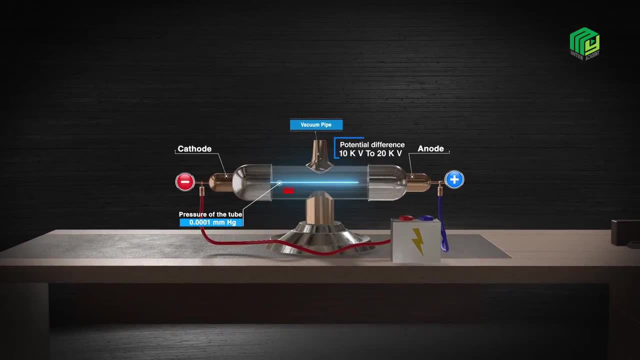 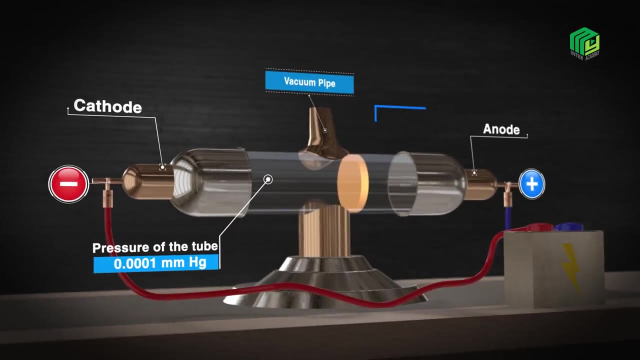 of glass tube. The rays emitted by the cathode travel towards anode. The attraction of rays towards anode reveals that the rays carry negative charge. Properties of the Anode. Properties of cathode rays are: 1. When any object is placed in the path of the cathode, 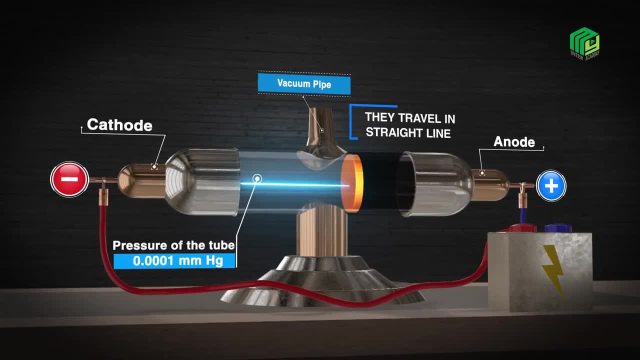 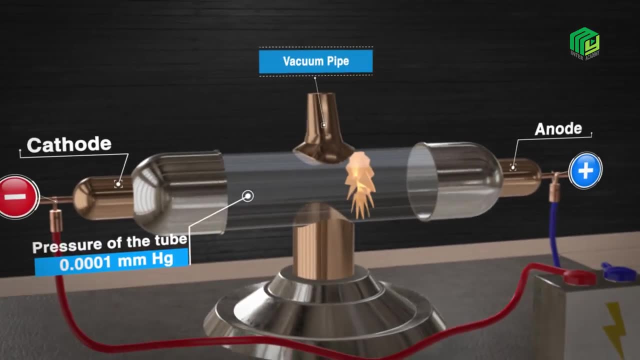 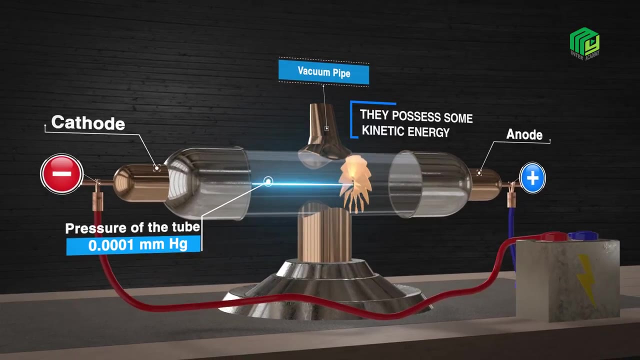 rays. these rays cast shadows. This shows that cathode rays travel in straight line. 2. When a wheel was placed in the path of cathode rays, the wheel rotates. This shows that rays consist of some particle and some kinetic energy. 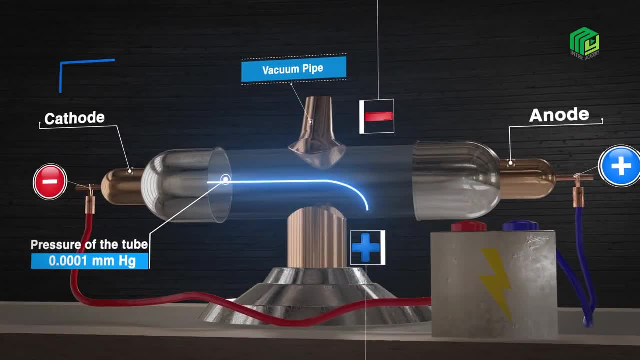 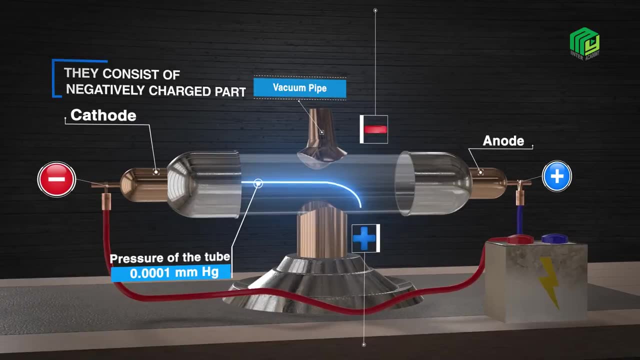 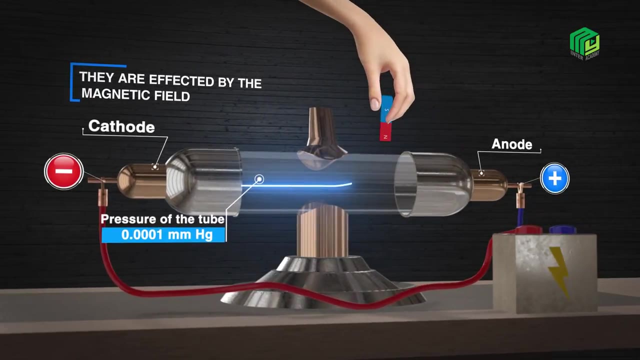 3. In the presence of an electric field, the rays are deflected towards the positive plate. This confirms that cathode rays consist of negatively charged particles. 4. In the presence of a magnetic field, the rays are deflected. This shows that the cathode 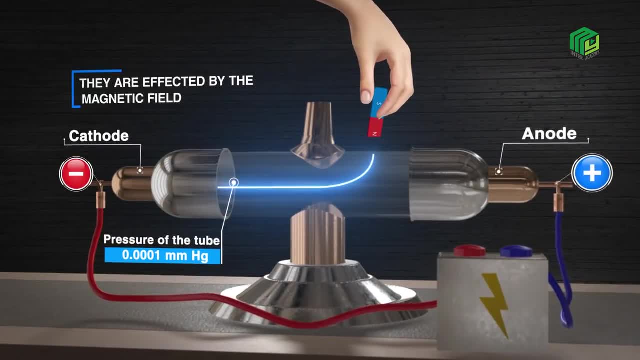 rays are affected by the magnetic field. 5. In the presence of a magnetic field, the rays are deflected towards the positive plate. 6. In the presence of a magnetic field, the rays are deflected towards the positive plate 7.. In the presence of a magnetic field, the rays are deflected towards the positive plate. 8. In the presence of a magnetic field, the rays are deflected towards the positive plate. 9. In the presence of a magnetic field, the rays are deflected towards the positive plate. 13. In the presence of a magnetic field, the rays are deflected towards the positive plate. 14..